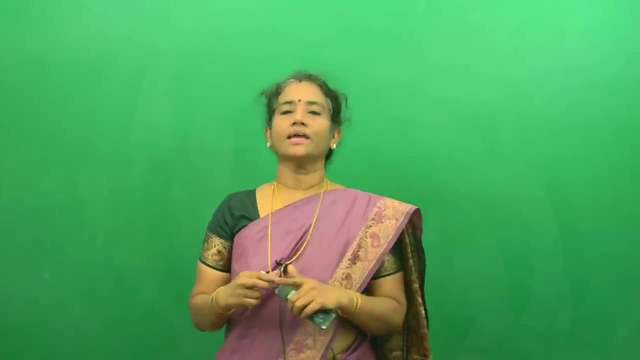 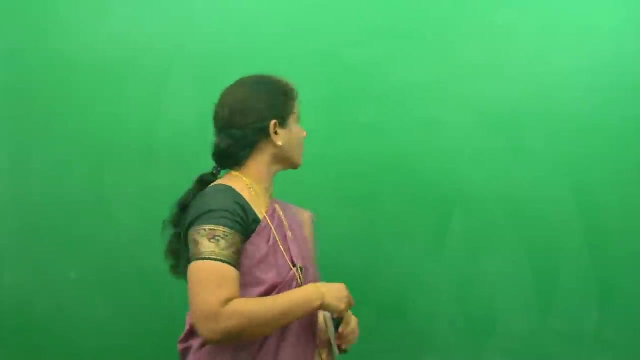 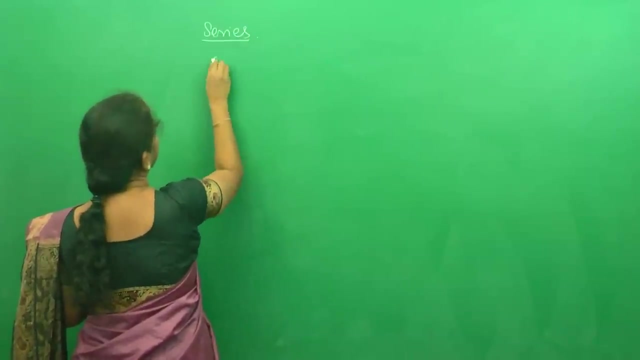 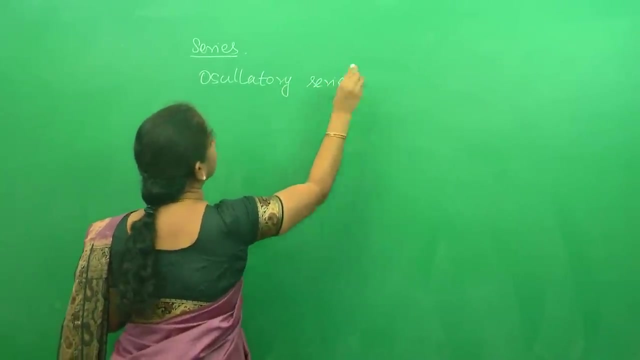 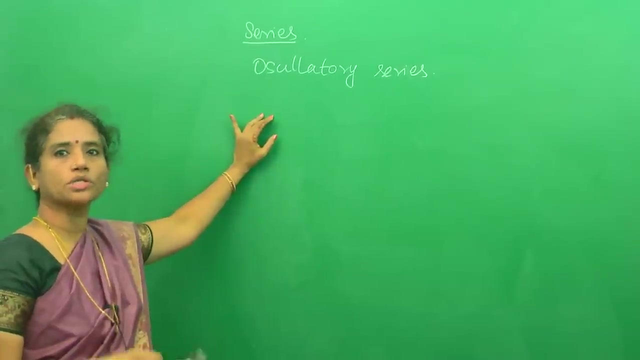 Hi everybody. in this session we are going to discuss the convergence or divergence of an oscillatory sequence. You clearly know, alternating oscillating series means one term will be positive, next term will be negative, next will be positive. it will be oscillating. 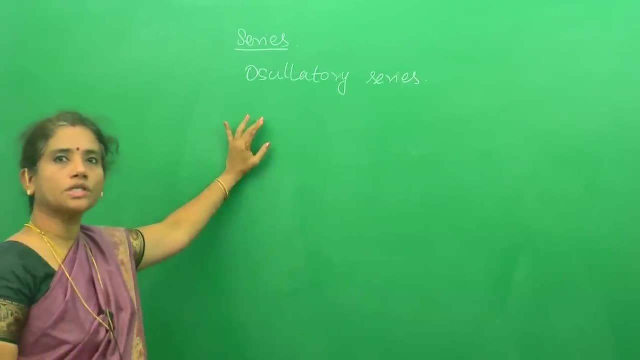 So even first term can be negative, second is positive, third is negative, fourth is positive. like that it will go on. So we are going to discuss the convergence or divergence of an oscillatory series. ok, For this we are going to use Leibniz test. 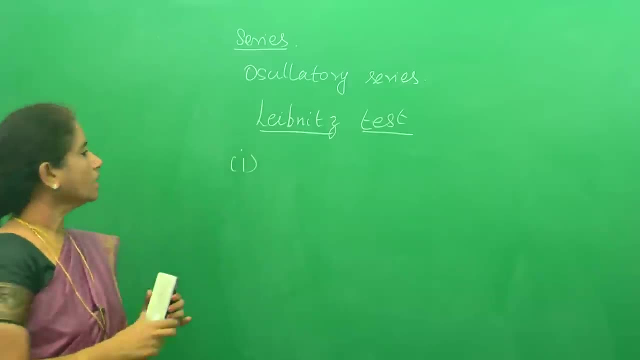 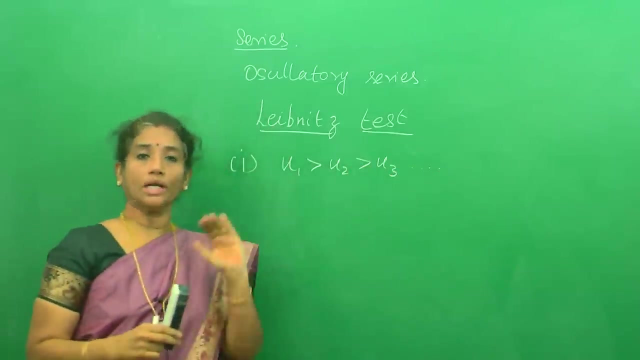 The test has two steps. The first step is: you are supposed to change the oscillatory series. So you are supposed to change the oscillatory series. So you are supposed to check u1 is more than u2, more than u3, etc. Means only numerically. 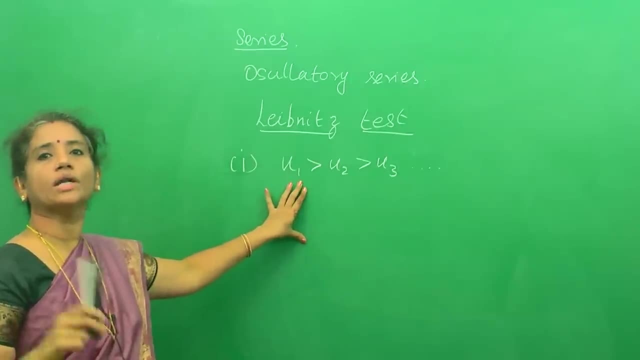 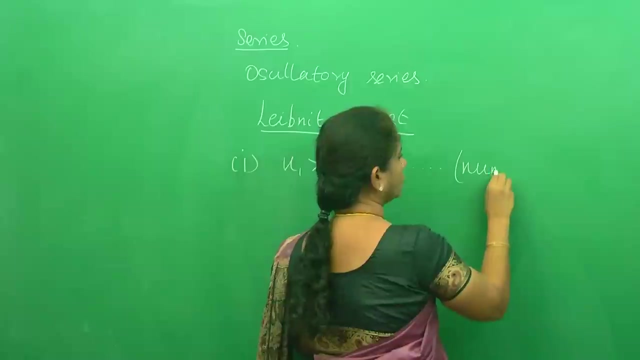 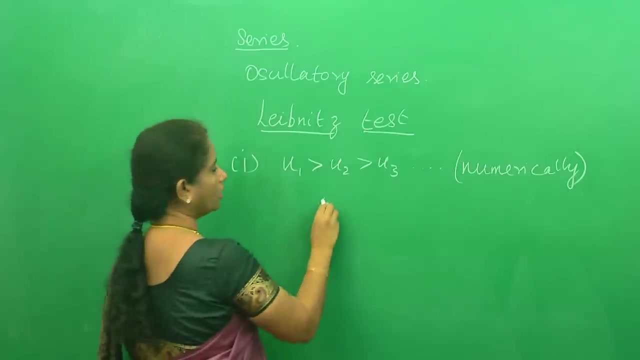 please be careful, because there is no meaning in comparing when one term is positive and one term is negative. ok, So numerically, just take u1, u2, etc. and you need to compare the first term with the second term, with the third term, etc. So generally we will be doing un. 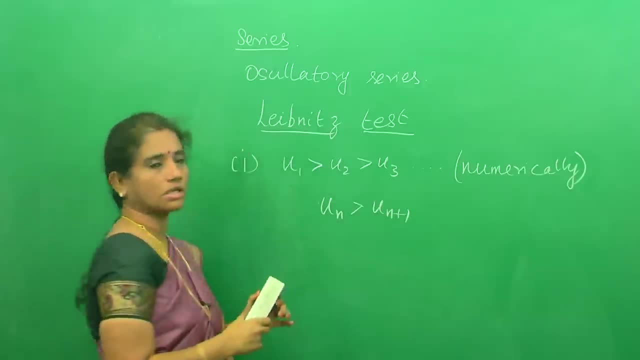 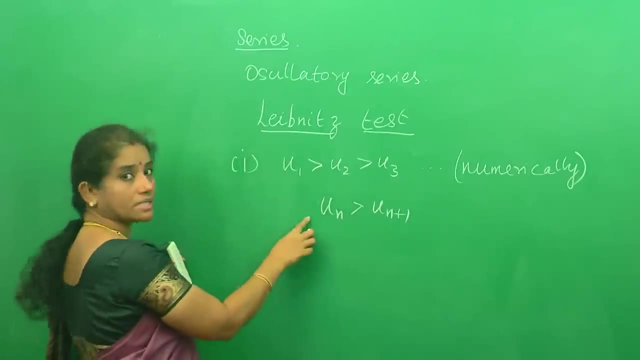 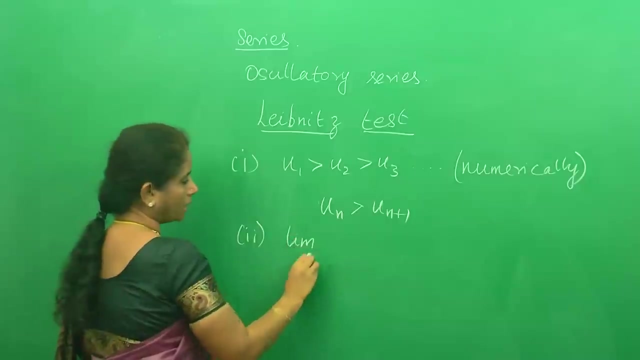 greater than un plus 1. we will be checking, that is all. because u2 is greater than un greater than u3 means un is greater than un plus 1.. After we do this, once this is satisfied- numerically is very important- once this is satisfied, the second step is very easy: limit. 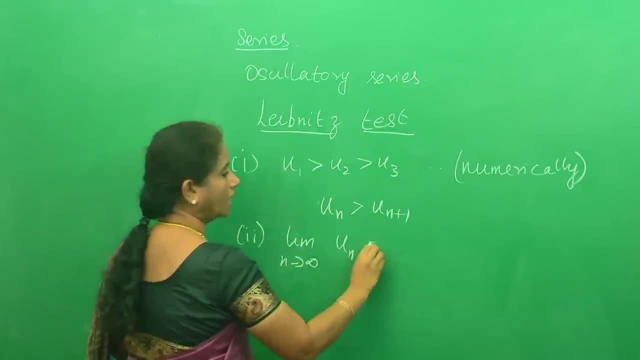 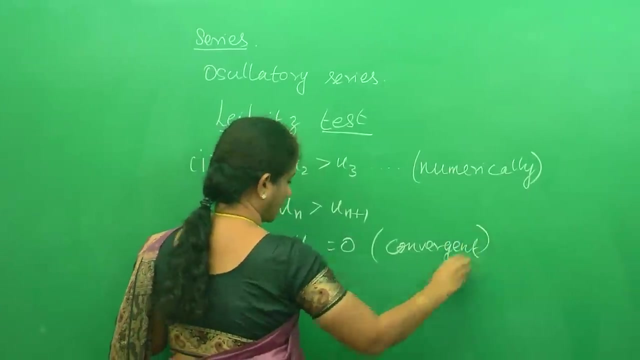 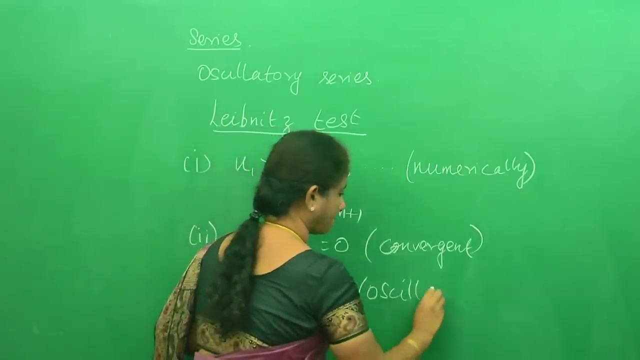 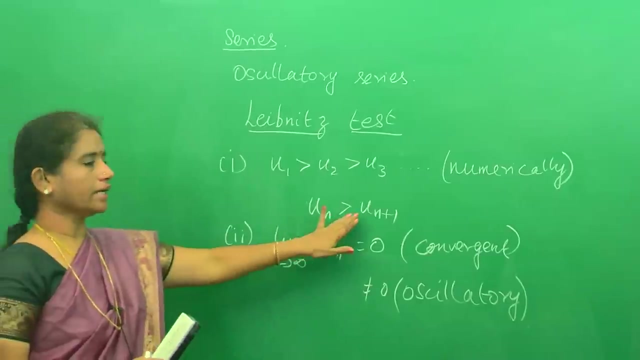 n tends to infinity un. you will calculate. if this is 0, the series is convergent and if this is not equal to 0, according to Leibniz test, the series is oscillatory. So there are two steps in this. one is un greater than un plus 1. we are going to check. 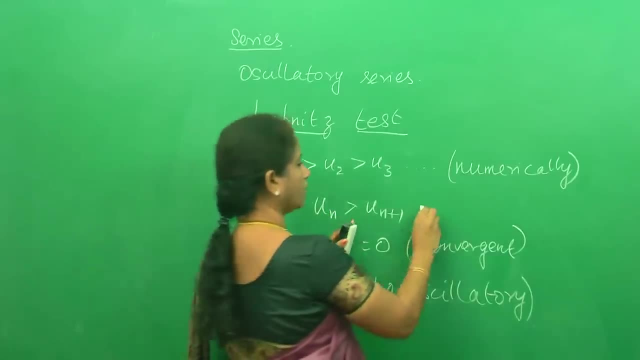 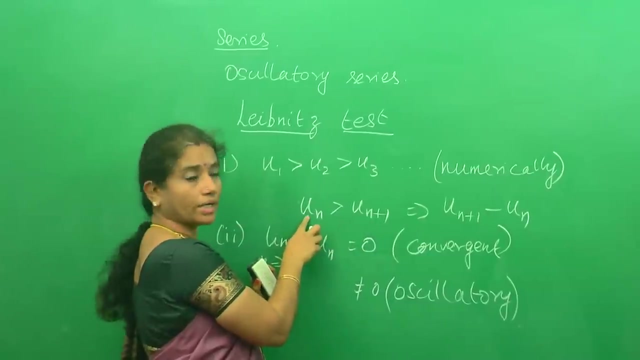 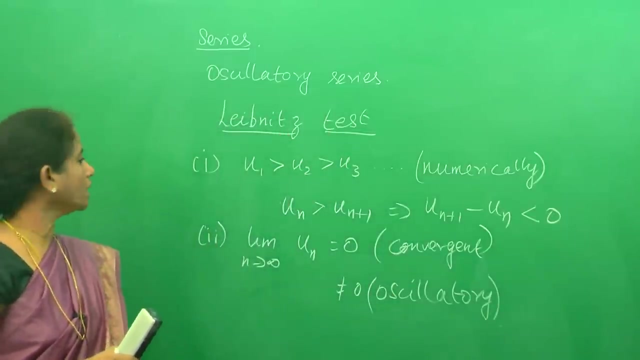 So for that, basically, we will be doing un plus 1 minus un. we will do So. this is the smaller quantity, this is a bigger quantity. So when you subtract this, this will become less than 0.. So we are going to check that and that is only numerically. we are going 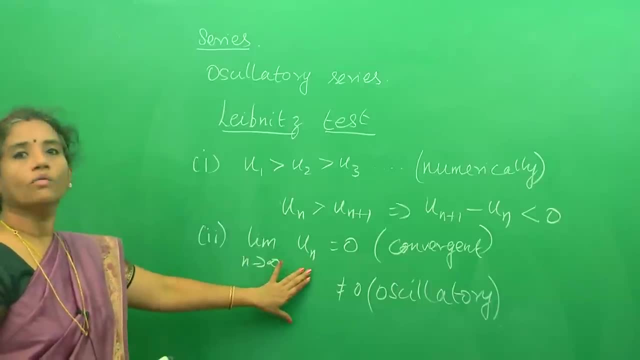 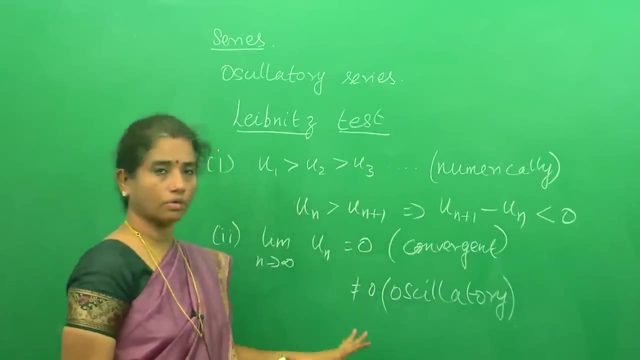 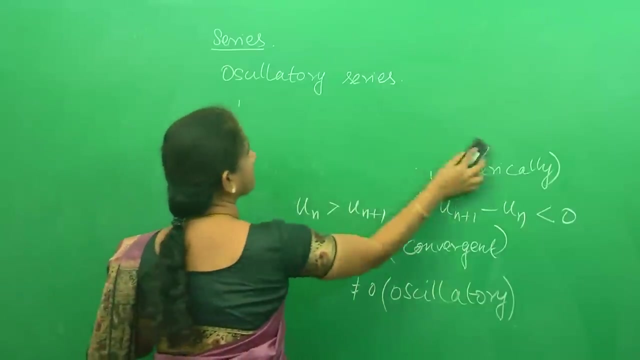 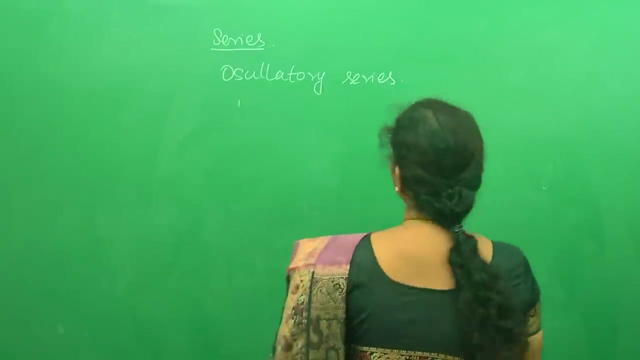 to check that. and second is limit: n tends to infinity. what happens to infinity? So happens to un. if it is 0, the series is convergent. any other number- positive, negative, anything, or infinity or whatever- the series is oscillatory. ok, now let us do few examples in this, so in 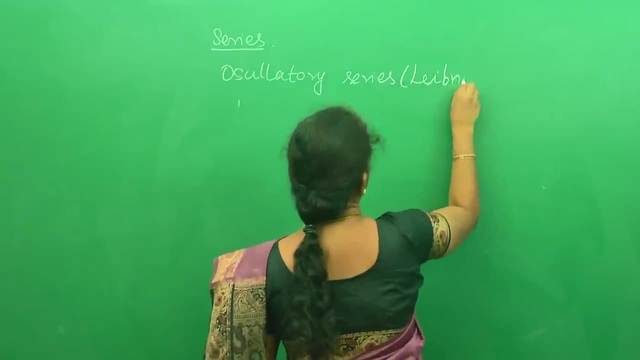 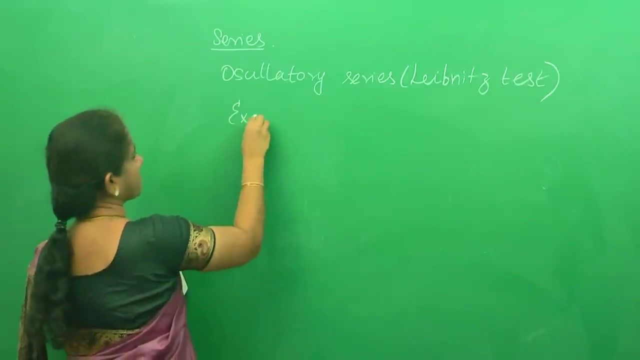 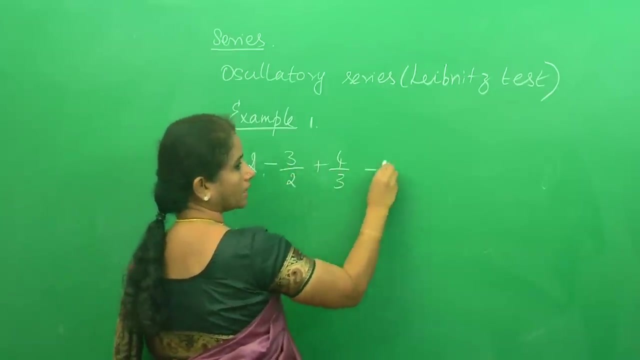 the oscillatory series. we are going to do Leibnitz test. ok, we will do few examples. first test the convergence of 1- sorry- 2 minus 3 by 2 plus 4, by 3 minus 5, by 4 plus, etcetera. 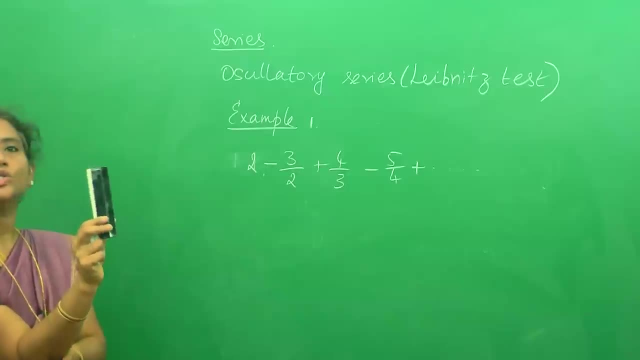 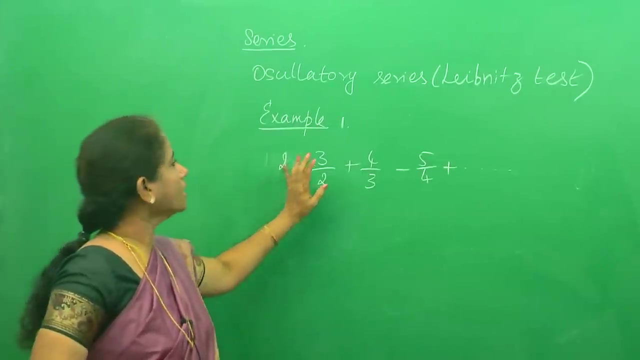 this has appeared in Anna University's test. ok In 2012 question paper. so we are going to find out the nth term, we are going to find out the n plus 1th term and then we are going to come back. un plus 1 minus un: what is the? 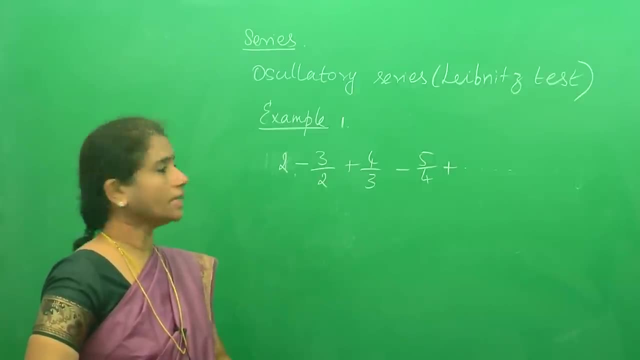 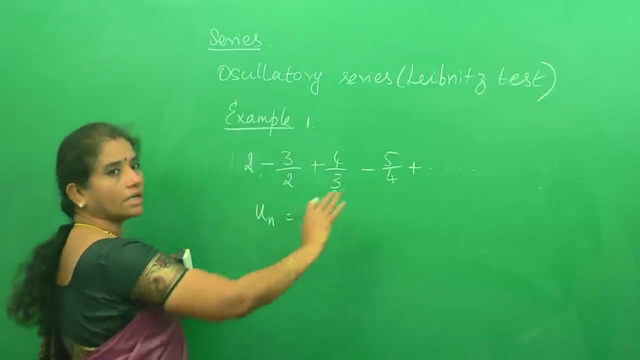 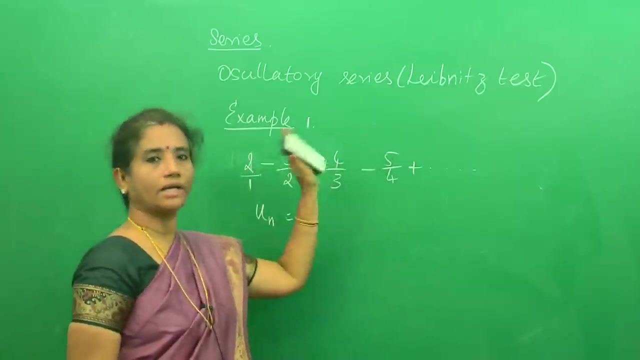 answer. after that we are going to find limit. n tends to infinity. what happens to un? ok, so as you have to write un, just look at the numbers in the numerator. this: I can write it as 2 over 1. if you look at it, you know 2, 3, 4, 5, like this: 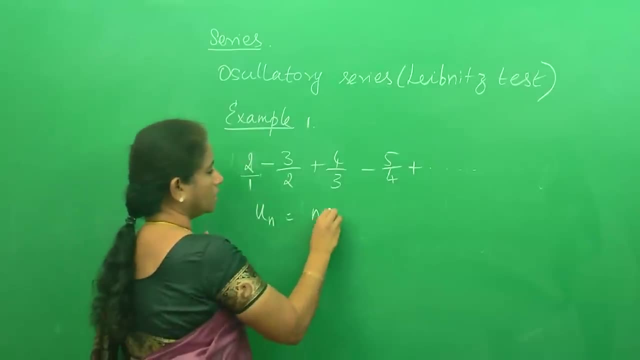 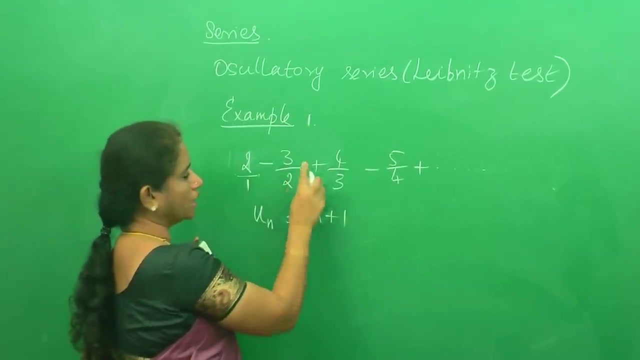 So the first term is 2. therefore it is going to be n plus 1. so when you put n is 1, you get 2, when you put n is 2, you get 3, when you put n is 3, you get 4, and it goes on coming to. 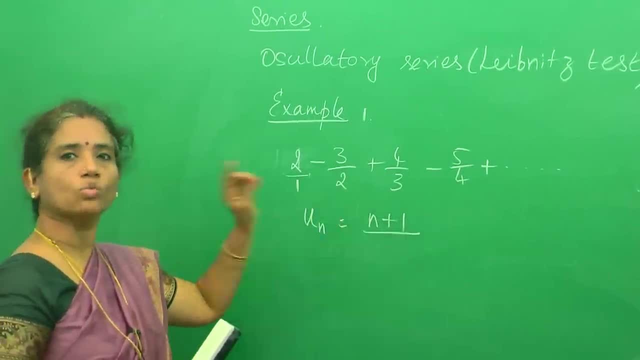 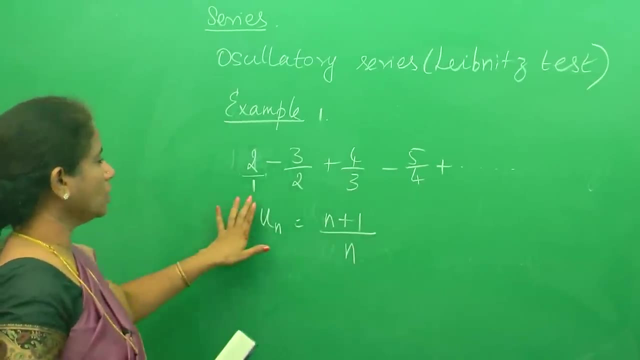 the denominator. you can see. denominator, each term is 1 smaller than the numerator. so this is 1, 2, 3, 4. so it is going to be n, even otherwise, we know 1, 2, 3, 4 means nth term is going to. 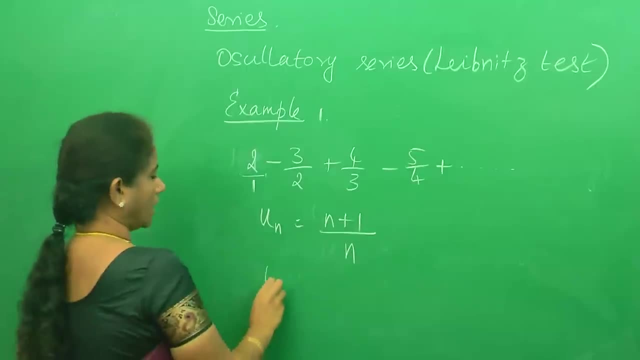 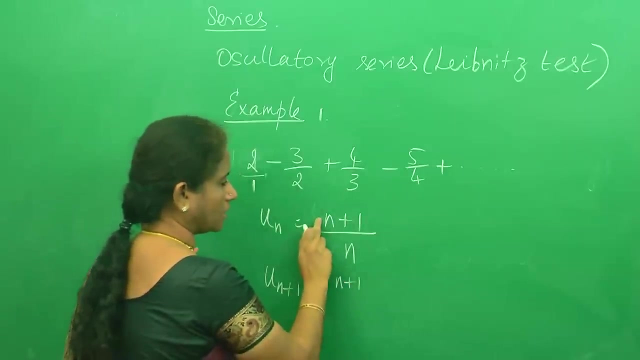 be n. So this is the un. now how do I write un plus 1? all n should be replaced by n plus 1. that is all. be very careful. n plus 1. this n is replaced by n plus 1. I just replace plus 1. 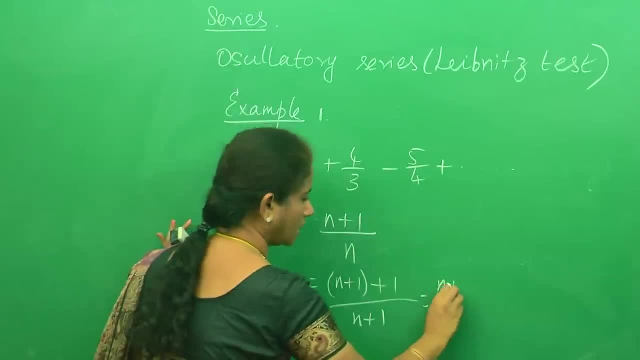 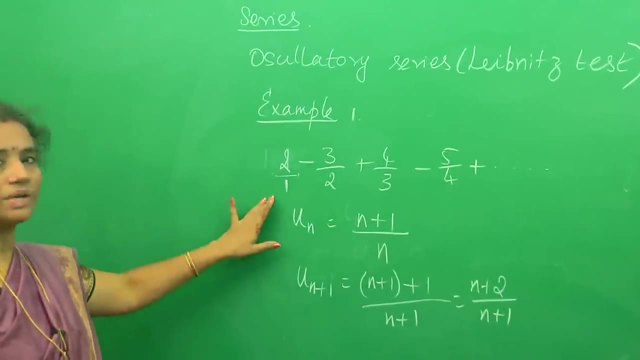 divided by this is n plus 1, which is nothing but n plus 2 divided by n plus 1.. So what is the first step in Leibnitz test? you are supposed to subtract these two and then check whether it is less than less than 1- sorry, less than 0- or more than 0, and then 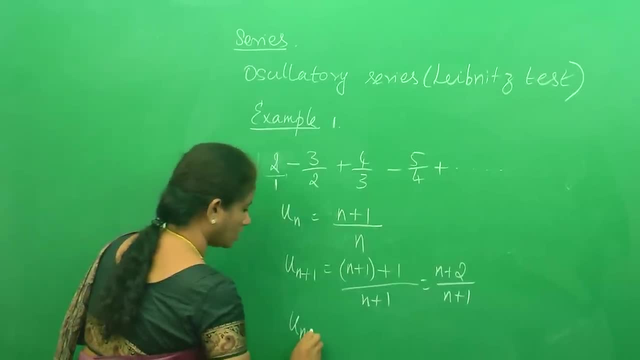 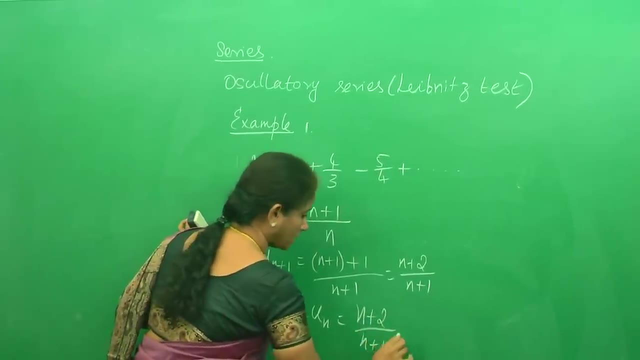 check whether it is less than 0 or less than 1.. more than 0.. So we are going to check un plus 1 minus un. So what is un plus 1?? It is very simple: n plus 2 by n plus 1 minus n plus 1 divided by n. You have to take LCM carefully. 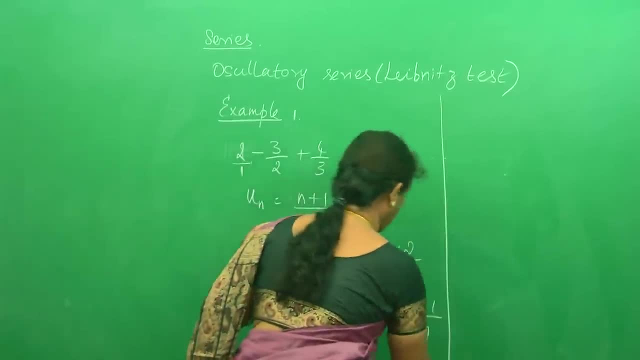 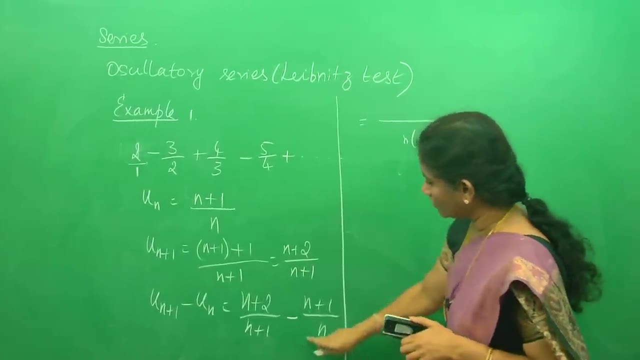 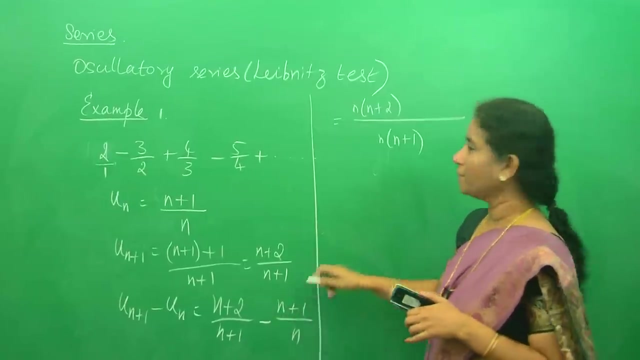 and when there is a minus, be careful with the negative sign. ok, So you know. the LCM is going to be n into n plus 1.. So this will be multiplied by n. n into n plus 2. minus, this term will be multiplied by n plus 1.. So minus n plus 1 times n plus 1.. Now I am. 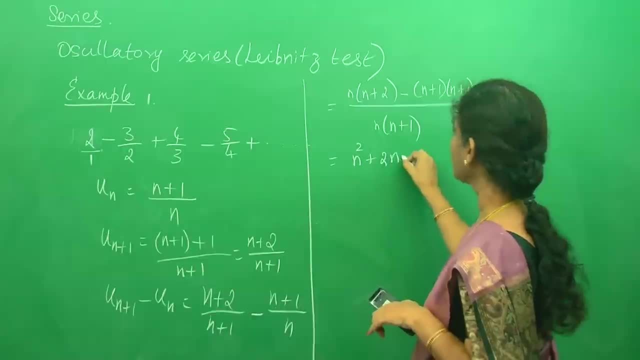 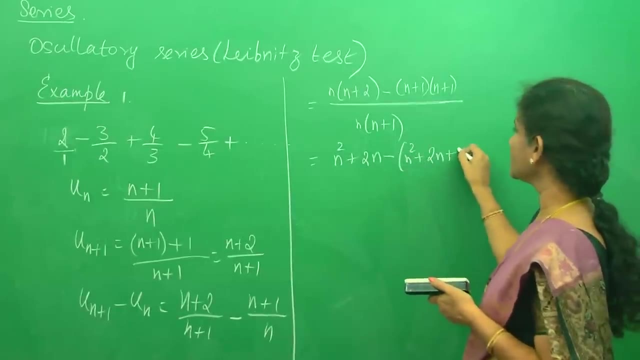 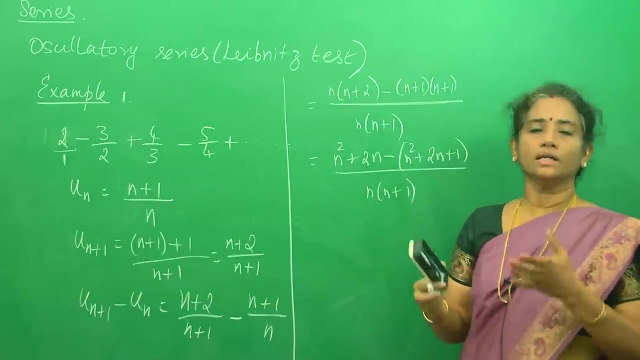 going to expand this n square plus 2n minus this is n plus 1, the whole square. So I can say n square plus 2n plus 1, divided by n, into n. Always remember n is positive because it is the term of the series t1, t2, t3, like that. 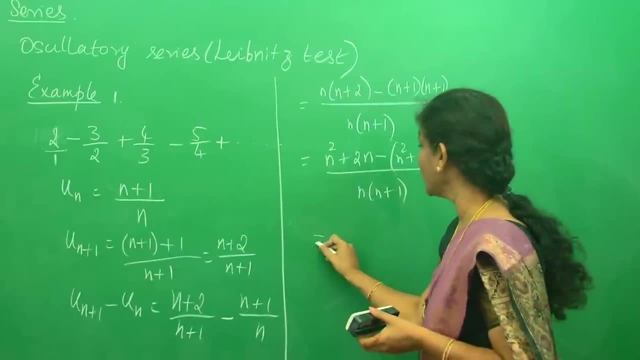 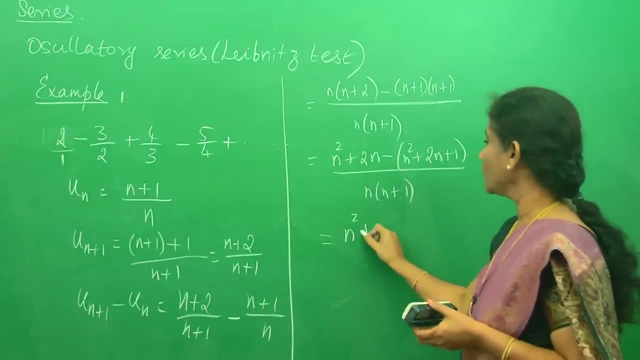 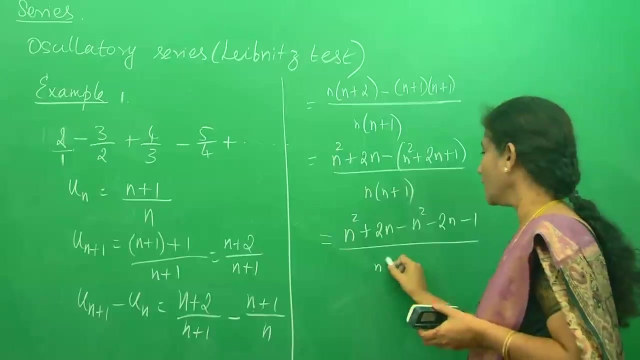 So n starts from 1 to 3 onwards, So it is a positive number. So be careful and write this bracket, otherwise you will miss out with this minus sign. So this is n? square plus 2n minus n? square minus 2n minus 1, divided by n into n plus 1.. You know this n? square. 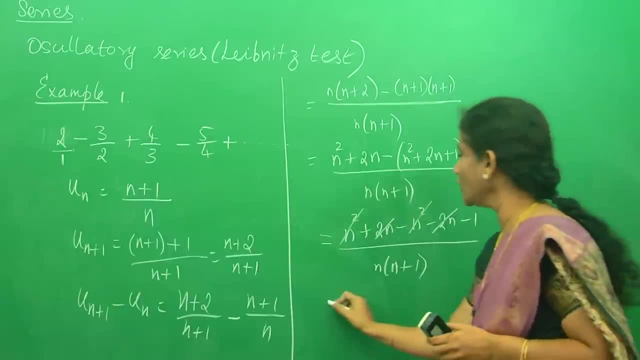 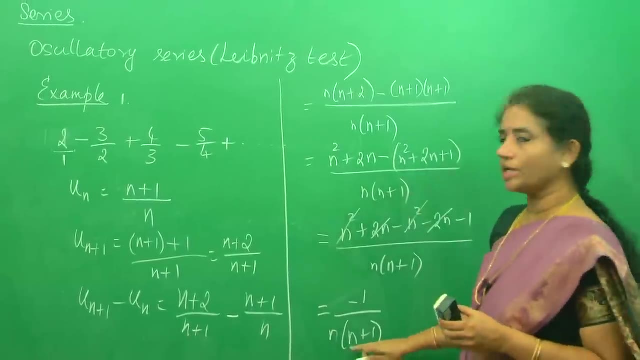 and n square cancels and this n square cancels. So this is n square plus 2n minus n square and n square cancels and this n square cancels and this n square cancels and this n square 2n will cancel with this 2n and you are left out with negative 1 over n into n plus 1, and you know. 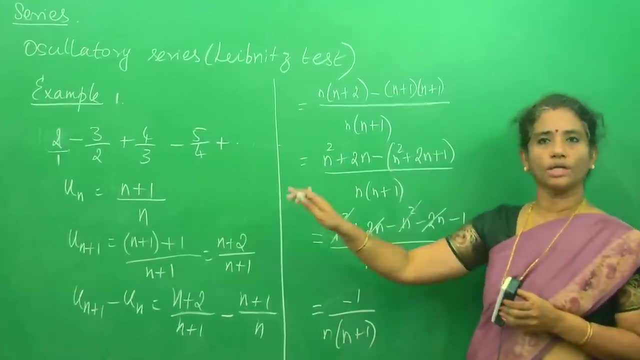 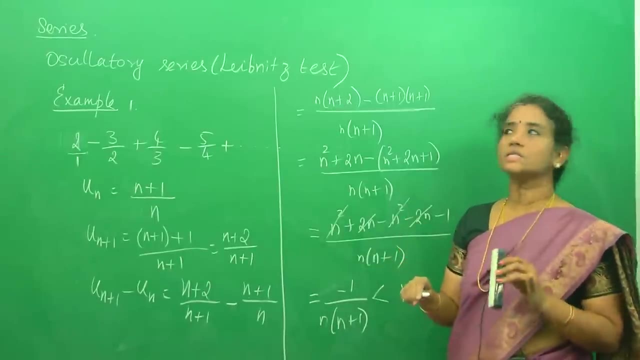 denominator is positive always, because n takes values 1,, 2,, 3, 1 plus positive and because minus 1 is there, this is less than 1.. So we have done the first step of Leibniz. test means the this term. 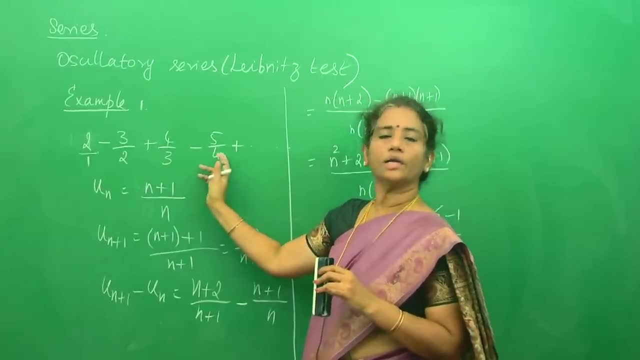 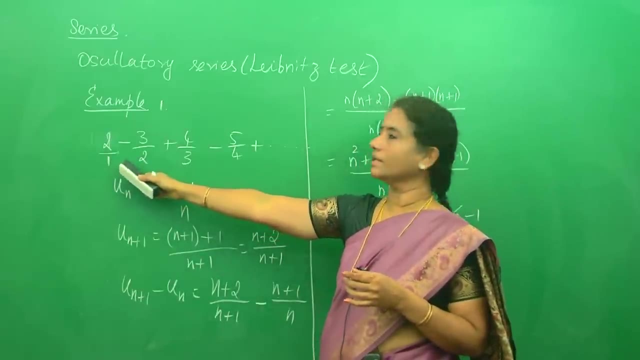 is smaller than this term. okay, You cannot compare it here. you have to compare it only with the nth term. okay, because looking at it you know 1 and a half is smaller than 2. but you cannot be saying that because that is just for the first two terms. You need to do un plus 1, un and then check. Now 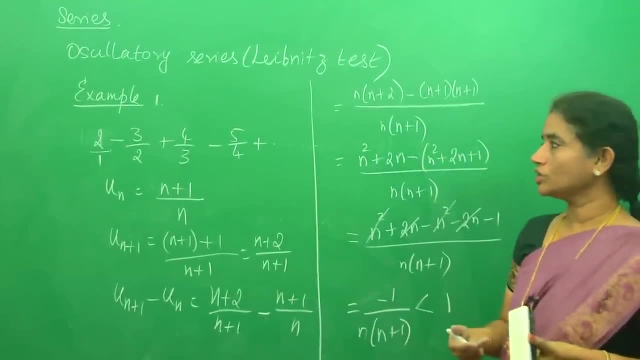 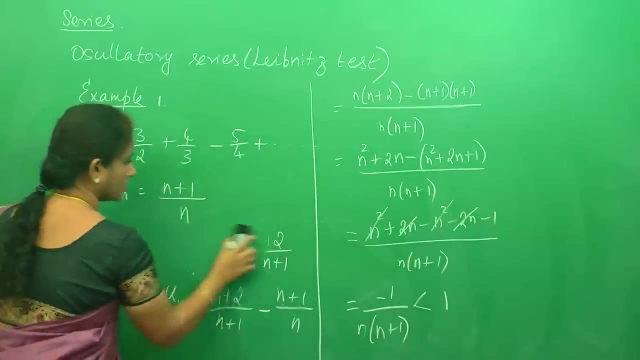 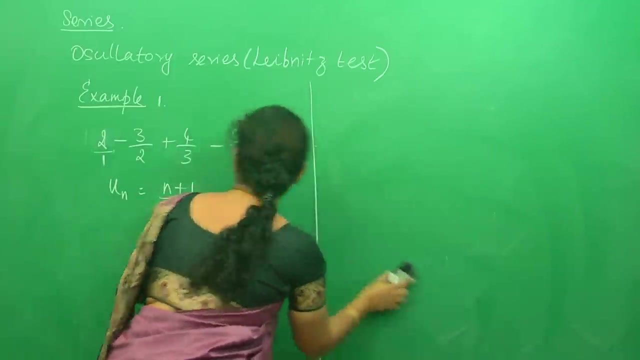 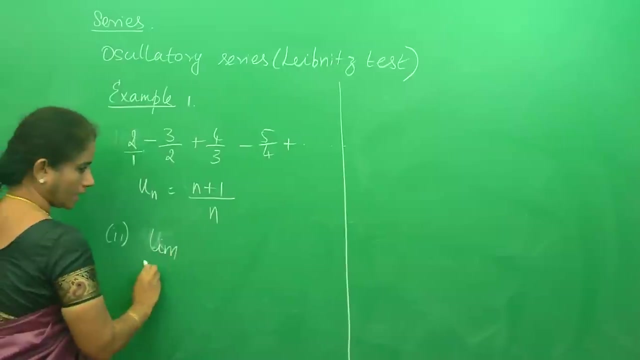 once the first step is over. it is very simple. I have to just check n tends to infinity. what happens to this? okay, So I am just having the nth term here. Now my second step. this is my second step. So this is: limit n tends to infinity, un. So limit n tends to. 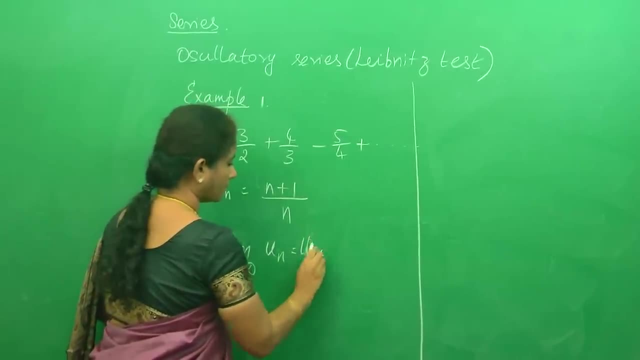 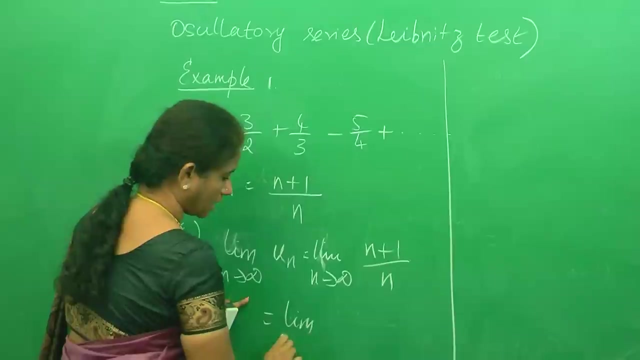 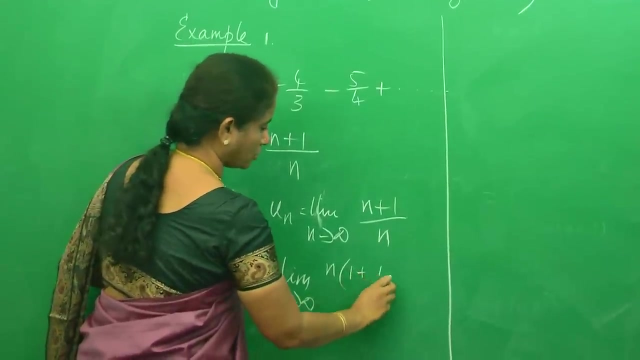 infinity. un will be limit n tends to infinity. n plus 1 divided by n, which is nothing but limit n tends to infinity. take the highest power of n from the numerator as well as the denominator. So, numerator, I took off. actually there is nothing in the 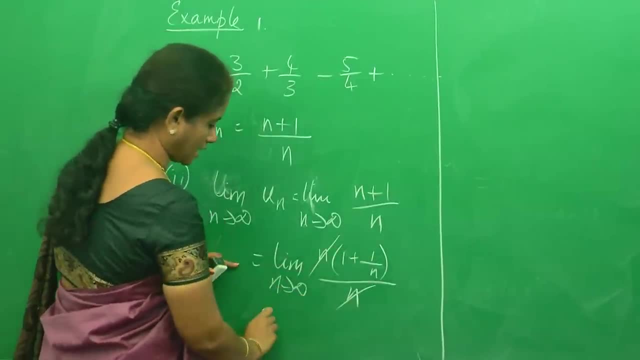 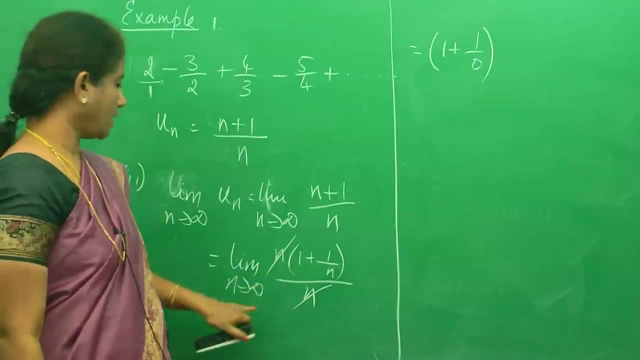 denominator. So I write it as it is. So this n gets cancelled. So what is your answer here? It is 1 plus 1 by 0, because 1 stays as it is. 1 by infinity is 0, you know that. So 1 plus z, sorry, 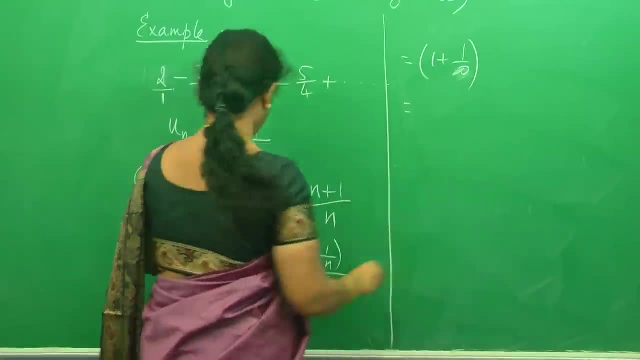 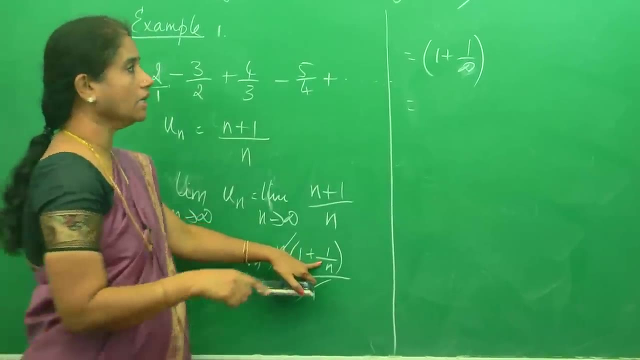 1 plus 1 by infinity. I repeat: limit n tends to infinity. When n goes to infinity, this becomes 1 by infinity, which is 0. So this is nothing but 1 plus 0, which is 1.. You know that you have to. 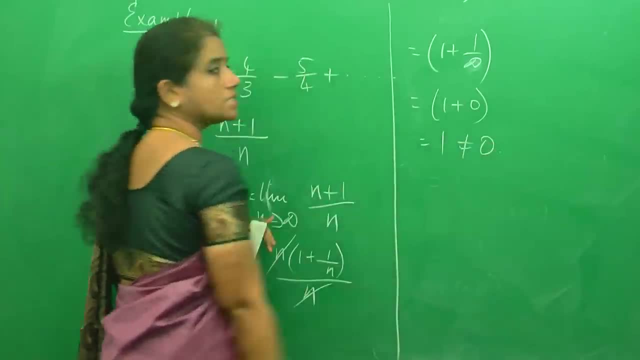 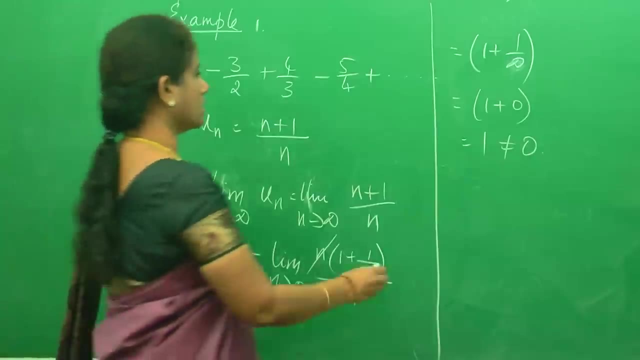 calculate. So I put just one small N here. So this is just 1 by infinity. So you now have llegaos. this is WITHIN infinity, So the we take out the ones that are going to be aн. So these are the就到, So what I call the LED ray, you can see, one of them is 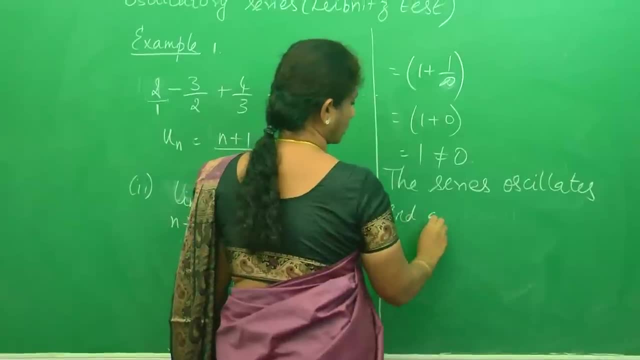 Gaddadi grid. So we just multiply all of this by Gaddadi r, you can see. even if I exchhhh 1 non secant value, the of this is L. I am not going to do that point because this is the. 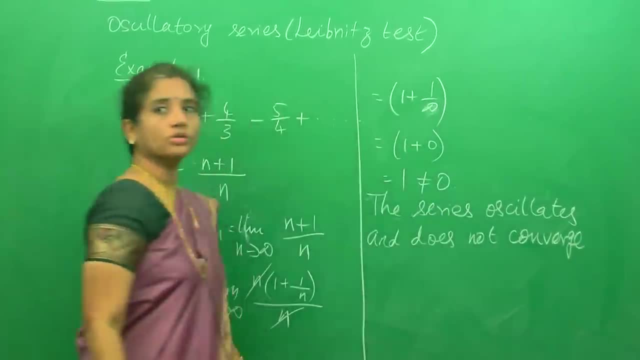 heat of the rayish. So the heat is the gamma volume of the ring, of the vlogging ring, ekta. So this is not equal to 0. very clearly, therefore, the given series oscillates. you cannot say it is convergent. and because this value is not equal to zero, okay, So you will conclude the series oscillates and it does not converge. So 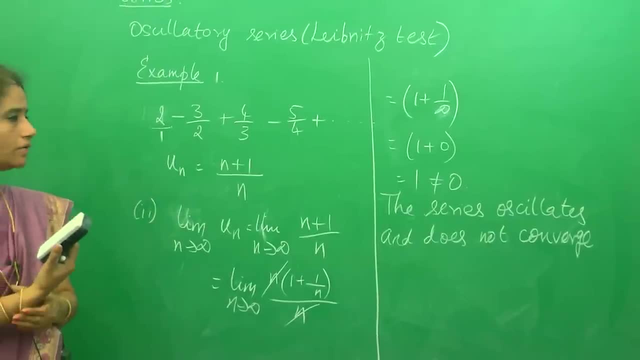 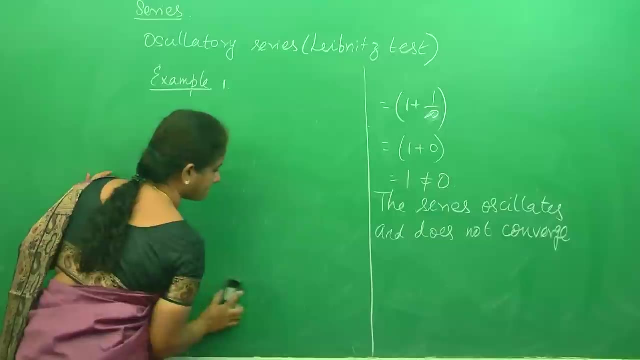 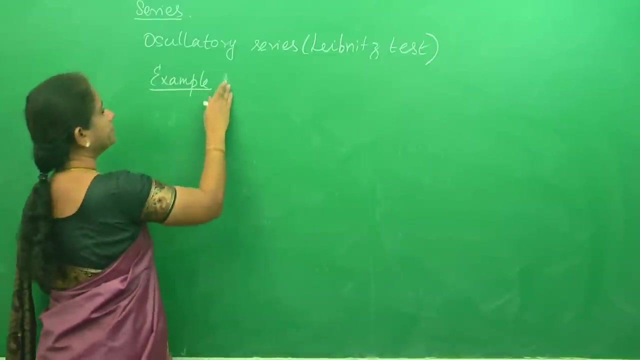 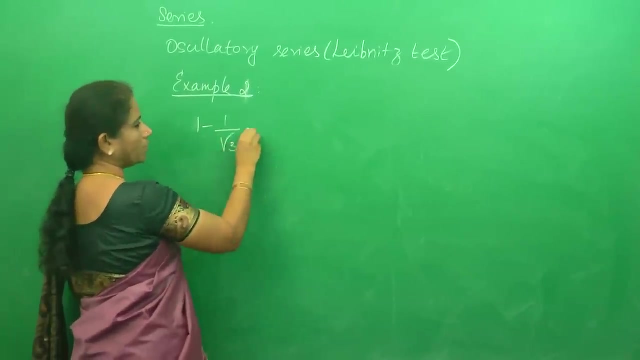 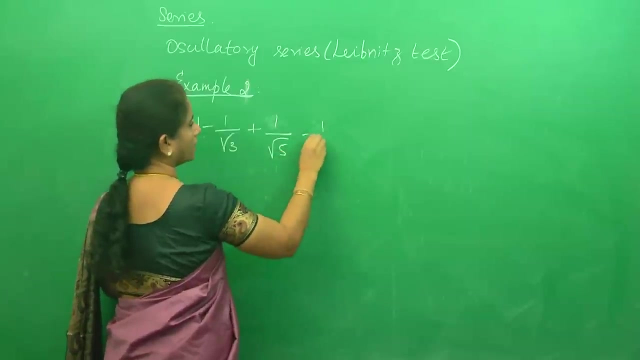 test you are going to identify whether the series is convergent or not. okay, We will do two more problems in this. Now we are going to test the convergence of 1 minus 1 by root, 3 plus 4 minus 1 by root, 5 minus 1 by root, 7 plus 1 by root, 9 minus, etc. This 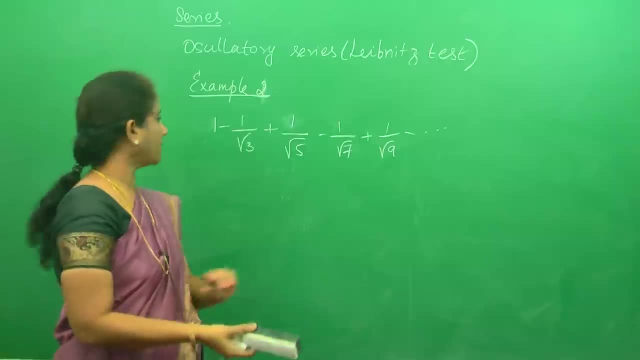 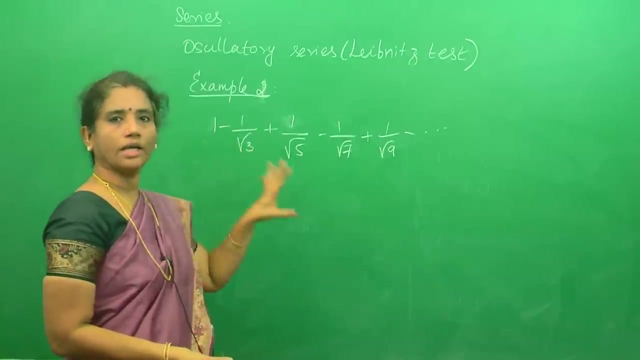 has appeared in an University Mail 2013 paper. So now you have got the series now and you can see the terms are oscillating. okay, Now we are going to write the nth term. So what is the nth term here? Numerator is all 1, okay. 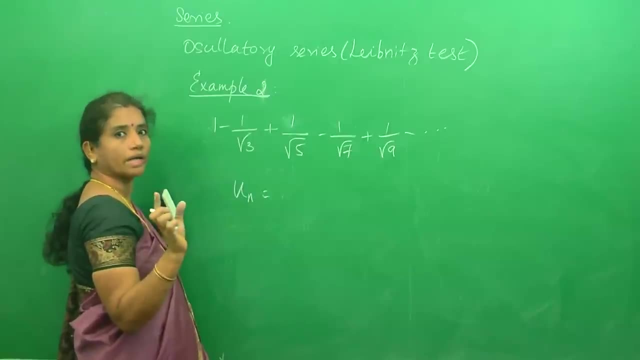 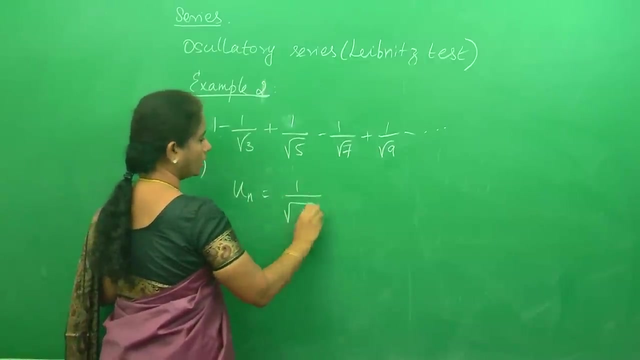 Please remember Numerically the nth term, So we do not care about the sign when you do this calculation. So this is your first step. So what is your un1 over root of? So this I can say it as: 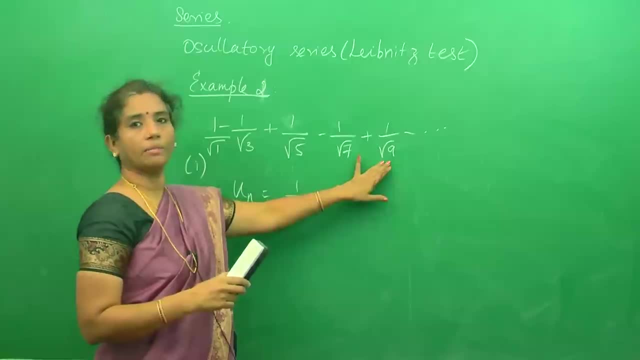 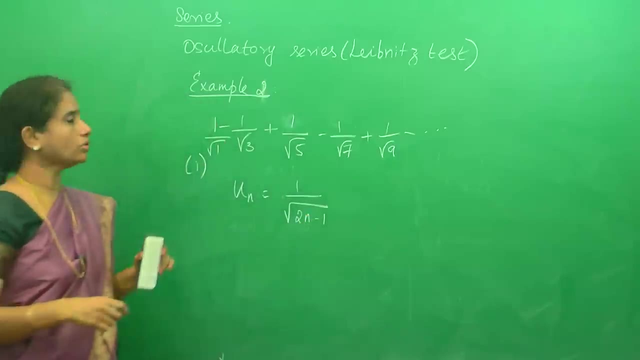 root 1,. okay, And you know, 1,, 3,, 5,, 7,, 9 means it is all odd numbers starting from 1.. So this is nothing but 2n minus 1.. So you can remember 1.. 2,, 4,, 6,, 8 means you will say: 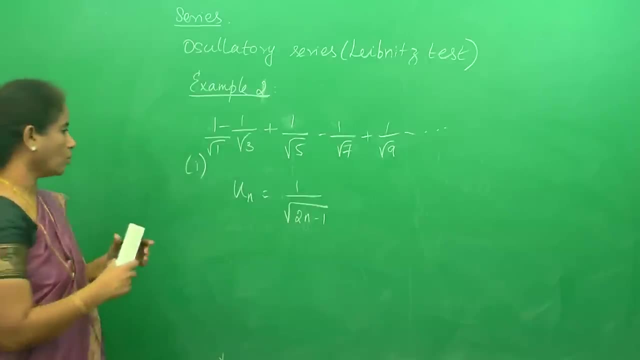 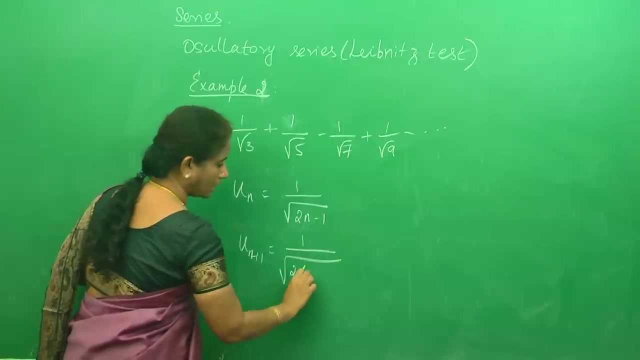 2n, 3,, 5,, 7,, 9 means you will say 2n plus 1.. And now I am going to write un plus 1.. As I told you in the previous example, in n plays you need to just put n plus 1 to get the un plus 1th term. okay, So this is. 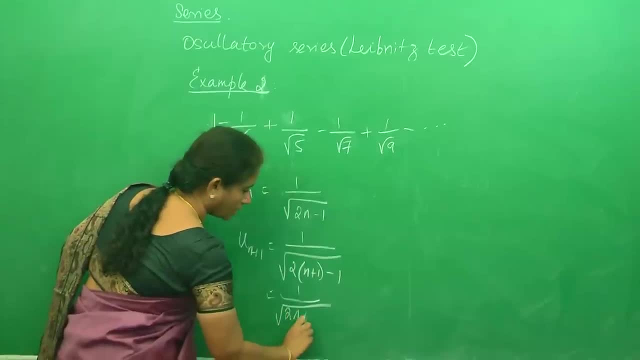 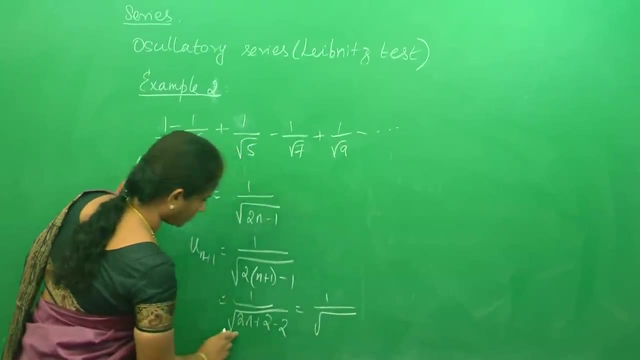 nothing but 1 by square root of 2n plus 2 minus 2n, which is nothing but 1 by square root of… I repeat, וש So…. So, when you want to write, un… u…, u…, u…. 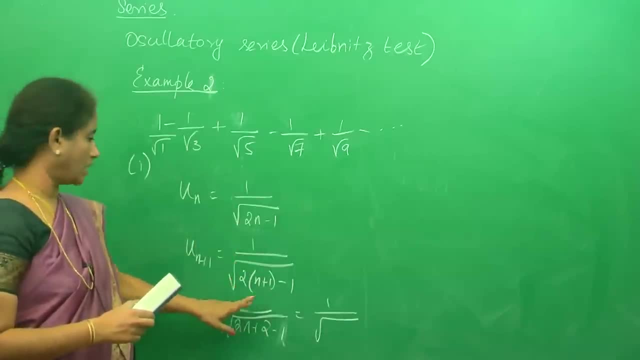 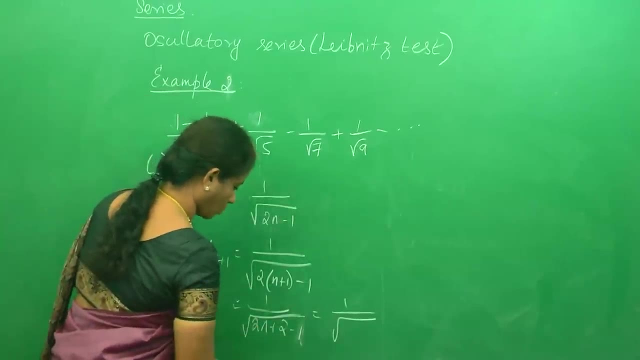 u… u… u… plus 1,. you just need to replace n by n plus 1.. So this is 2 into n plus 1.. So this becomes 2n plus 2 minus 1, and 2 minus 1 is 1.. So you get the answer as n plus 1.. So now I. 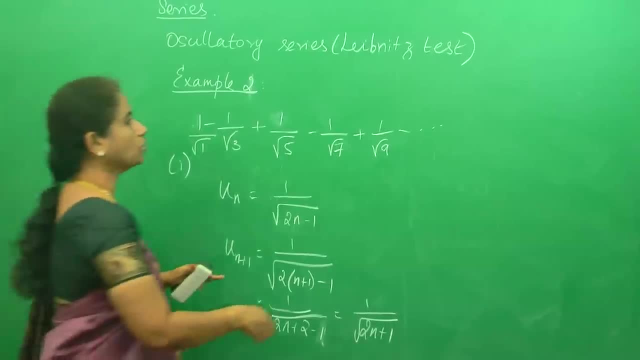 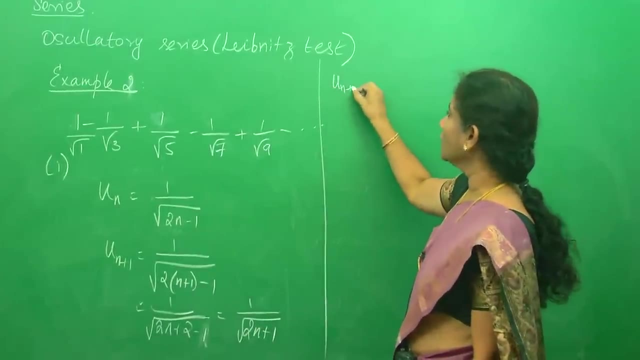 found un. I found un plus 1.. Now I just have to subtract and check if this is more or means what happens to the subtraction. un plus 1 minus un is nothing but 1 by square root of 2n plus 1. 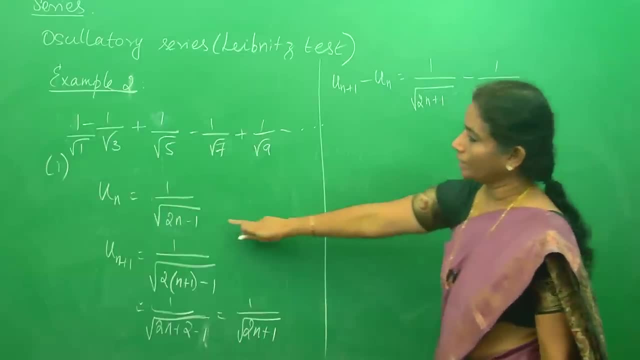 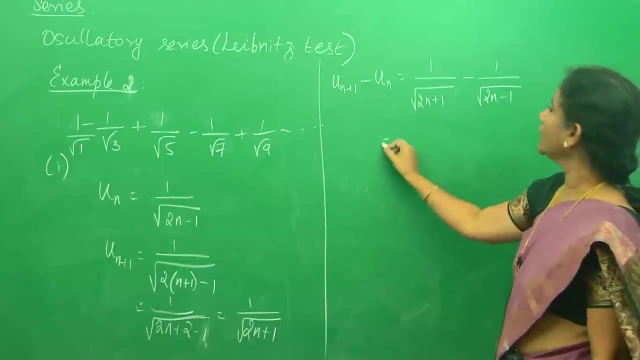 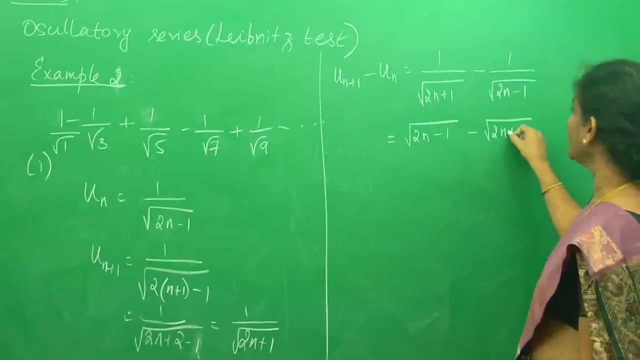 minus 1 by square root of 2n minus 1.. That is your un. this is your un plus 1. ok, 2n minus 1.. So now I take the LCM. this becomes square root of 2n minus 1, minus square root of 2n plus 1. 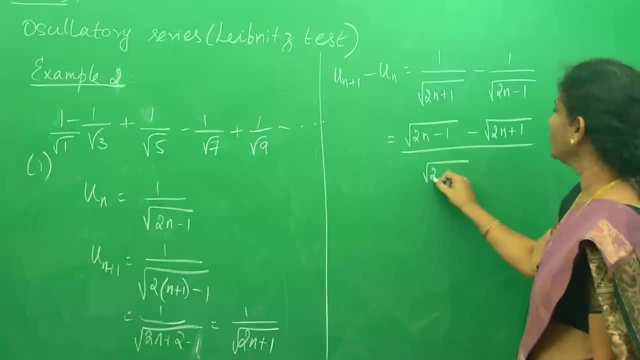 divided by square root of 2n minus 1.. So this is the subtraction. So this is the subtraction. So square root of 2n minus 1 minus square root of 2n minus 1 minus square root of 2n minus 1.. 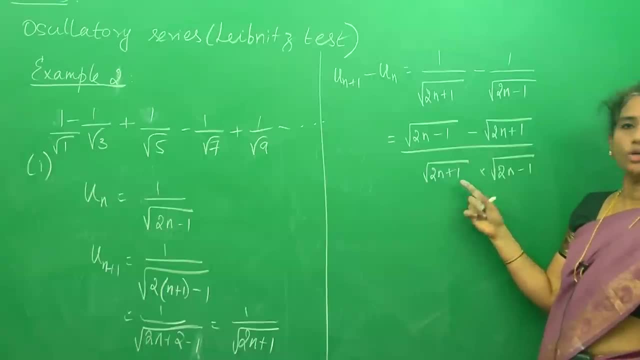 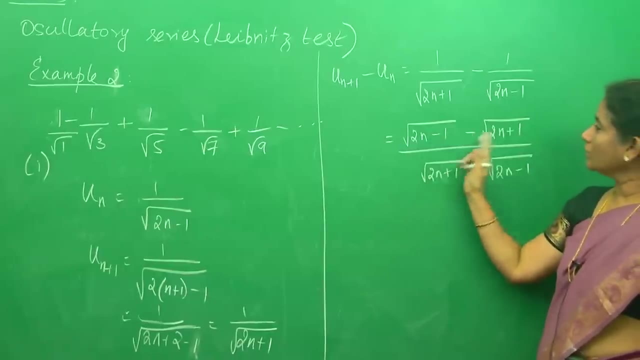 Just look at it. You know denominator is positive, clearly, you know, because n is 1,, 2,, 3, etc. Any value after 1 only means 1 and above only. you can take. Now, coming to this part, 2n minus 1 is 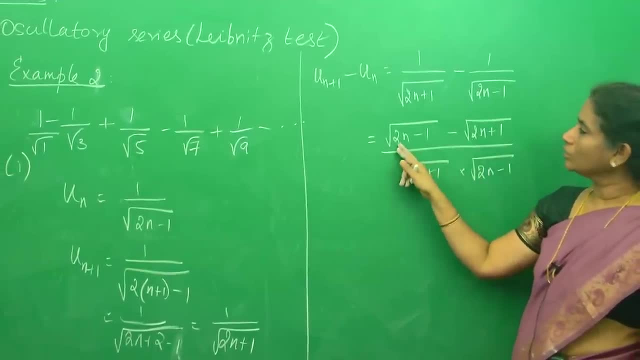 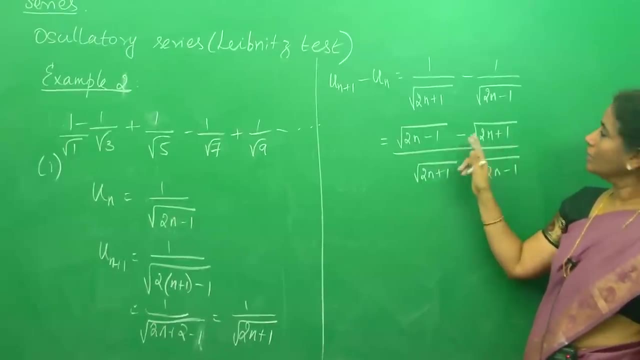 definitely smaller than 2n plus 1, because from 2n you are subtracting 1 here, but to 2n you are adding 1 here. ok, So this term is subtracted, So this is the subtraction, So this is the. 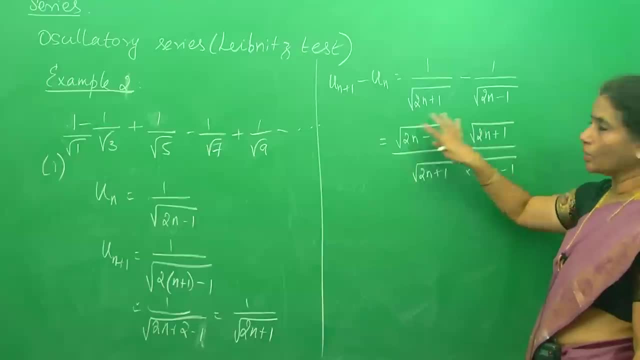 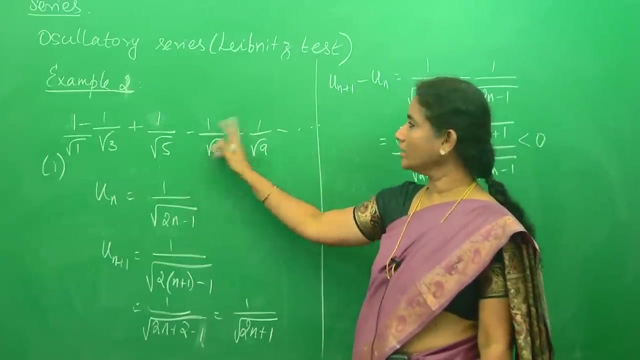 bigger one. So when you subtract a smaller number- sorry, when you subtract a bigger number from the smaller number, your answer is going to be less than 0.. So your first part of Leibniz test is checked means this term is smaller than this term. once again, you can look at it and check. 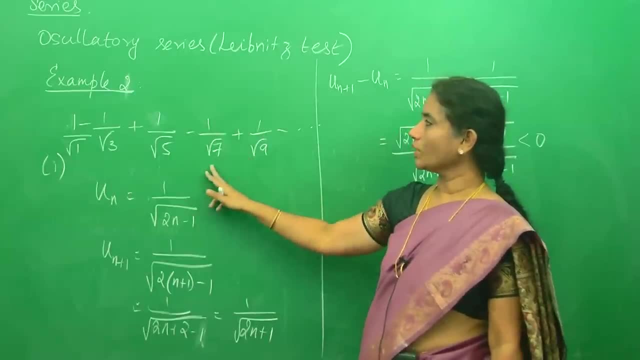 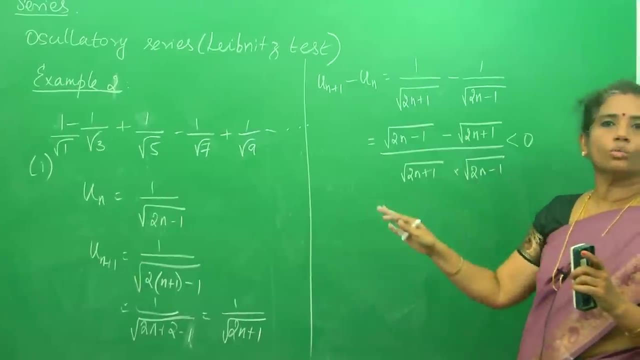 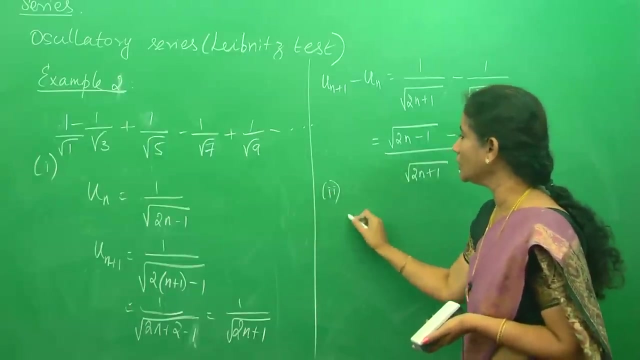 for yourself. this is 1 by 3, this is 1 by root 7. you know this is smaller, correct? ok? So just always think. when you get the answers, always go back to the question and just think whether you have done it correctly. ok, Now your second step in Leibniz equation: you are going to find limit. 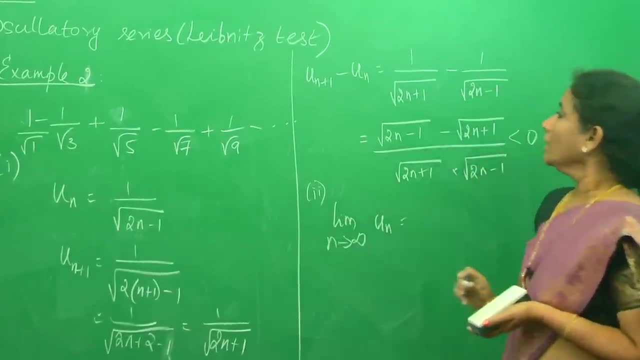 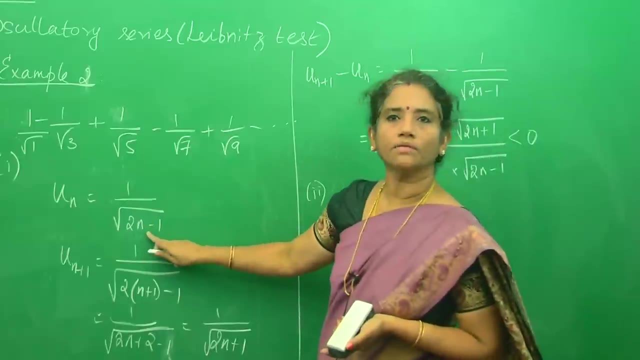 n tends to infinity, un. So let us do what is limit. n tends to infinity. un, which is nothing but un, is this is your un: 1 divided by square root of 2n minus 1.. So this is 1 divided by square. 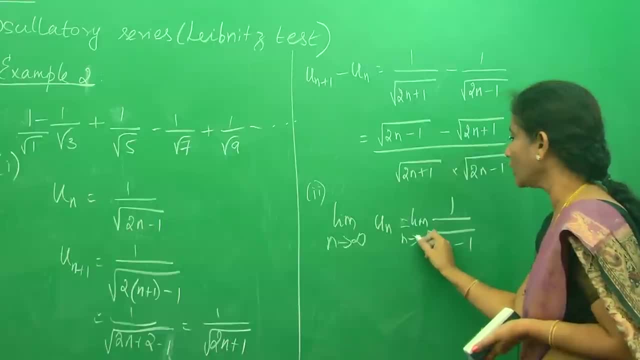 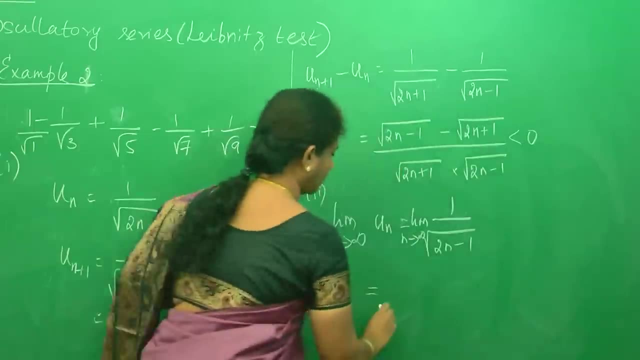 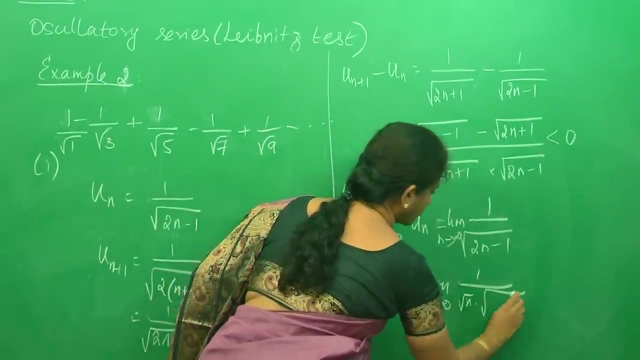 root of 2n minus 1.. For this you are going to check what happens. limit n tends to infinity. ok, As usual, take the highest power out, ok. So this is. limit n tends to infinity. 1 by square root of n into square root. 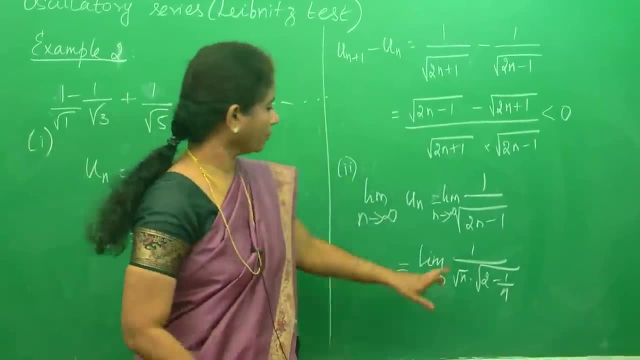 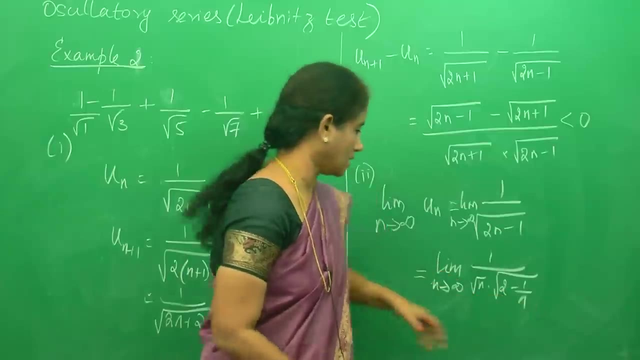 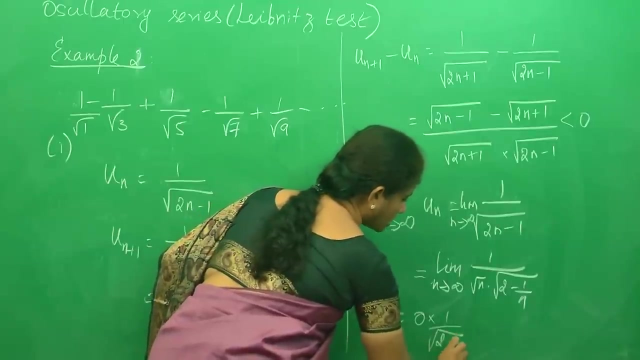 of 2 minus 1 by n. You know, when n goes to infinity, 1 by root, n goes to 0 and 2 minus this also becomes 0. So this is 0 times 1 by square root of 2 minus 0, which is 0.. So what happens now? each, each, the next. 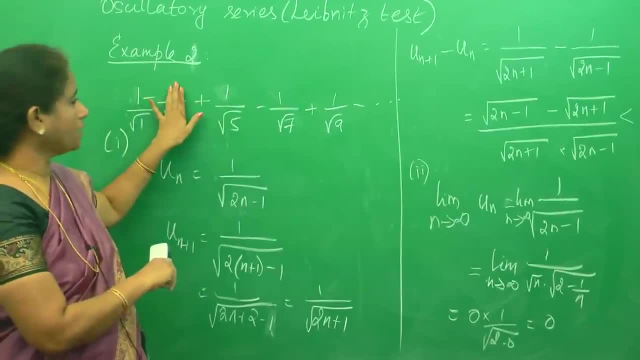 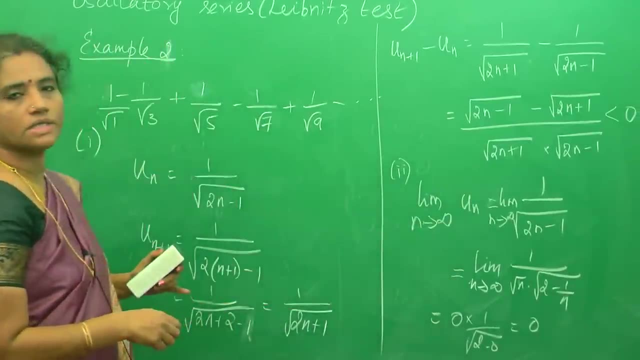 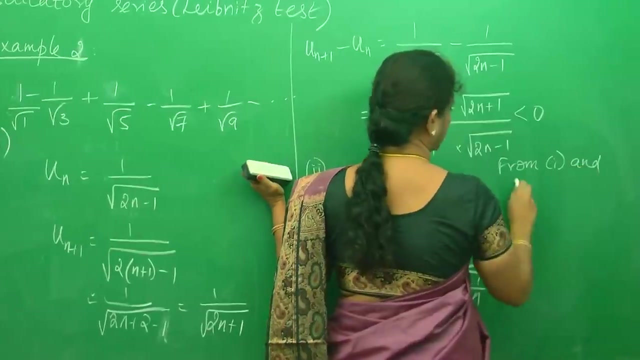 term is smaller than the previous term and the limit n tends to infinity. un also goes to 0 by Leibniz test. the given series is convergent. ok, So you can say from 1 and 2 by Leibniz test. 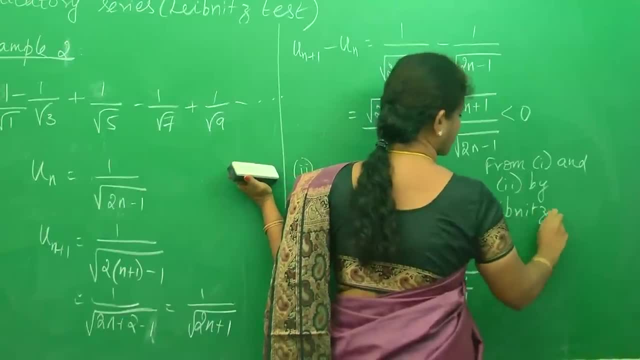 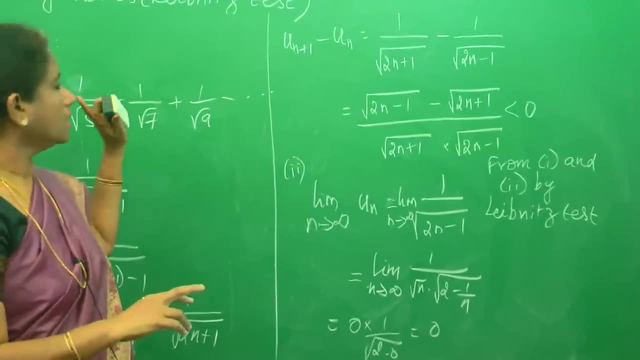 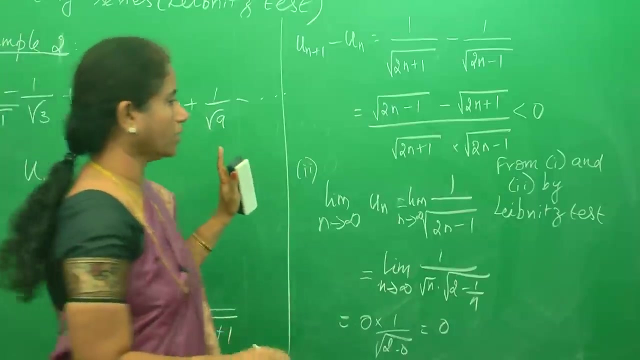 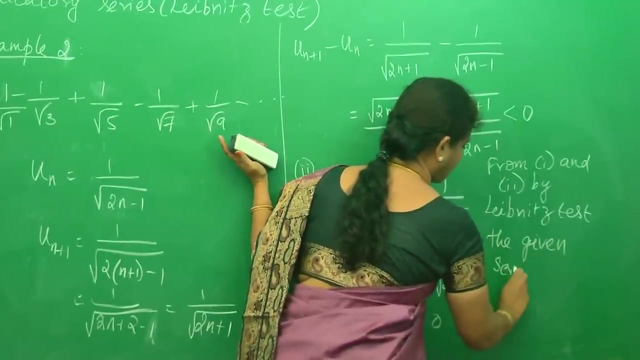 The series is convergent. always remember two things when you do Leibniz test. one is: take the numerical value for doing un and un plus 1.. Do not take the with the sign ok from 1 and 2 by Leibniz test. the given series is convergent. 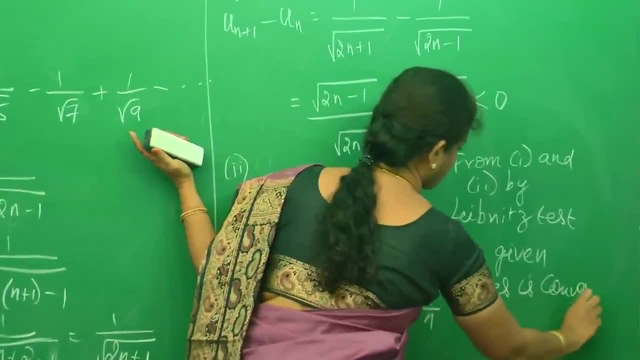 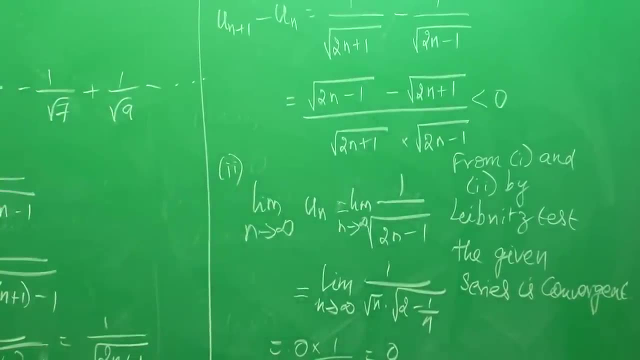 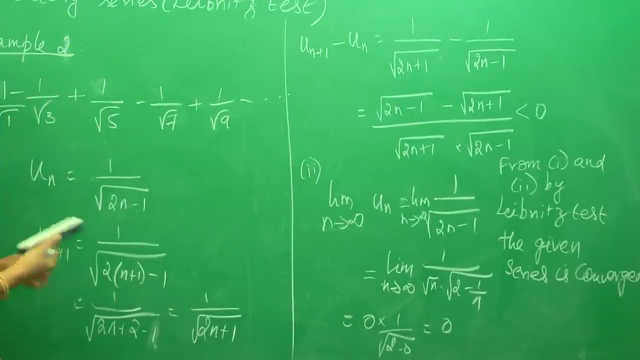 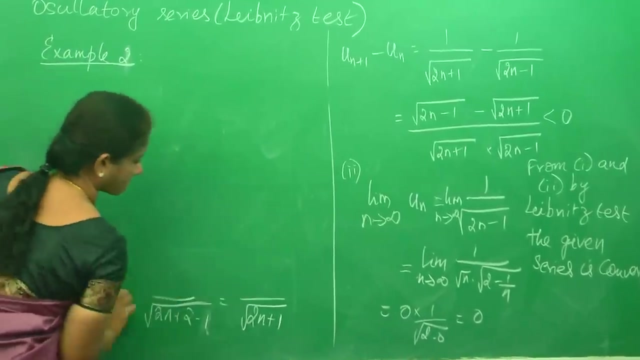 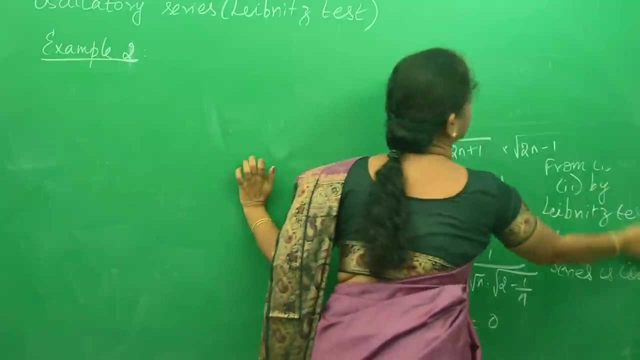 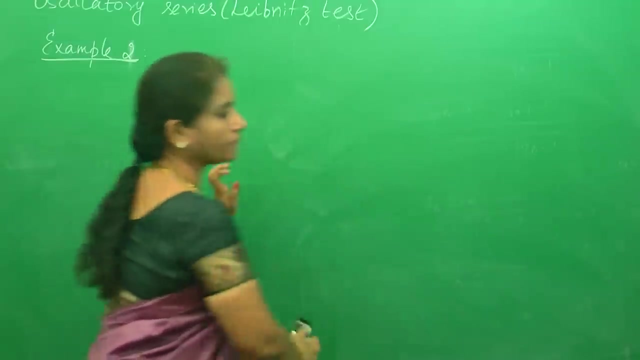 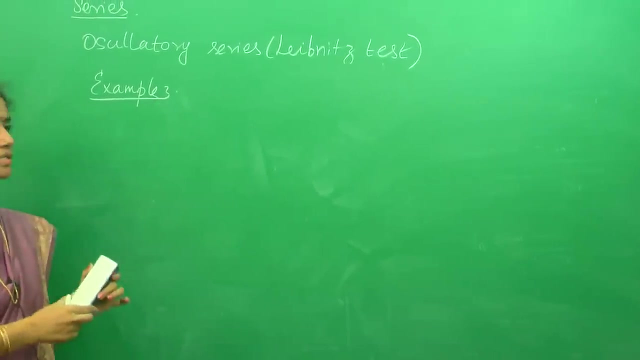 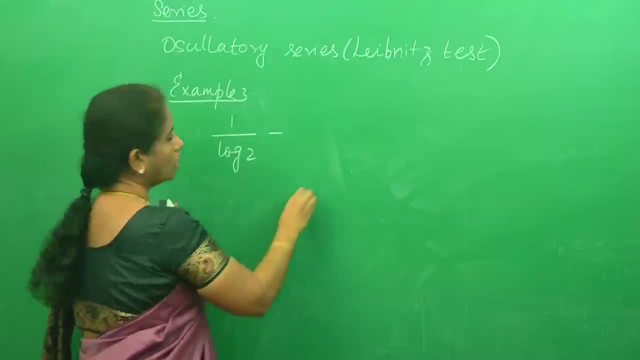 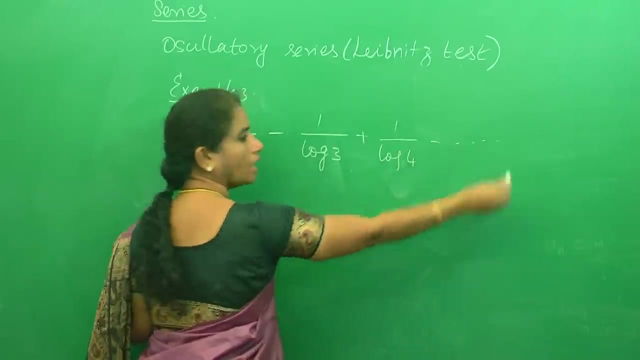 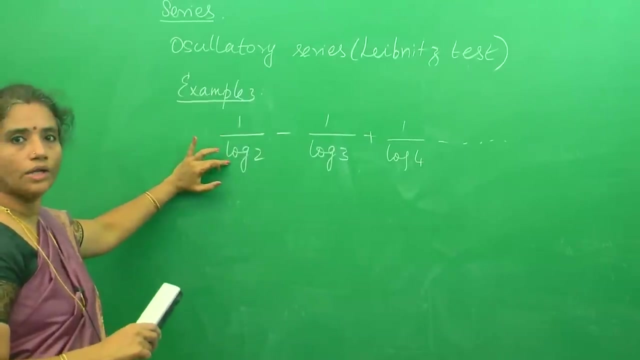 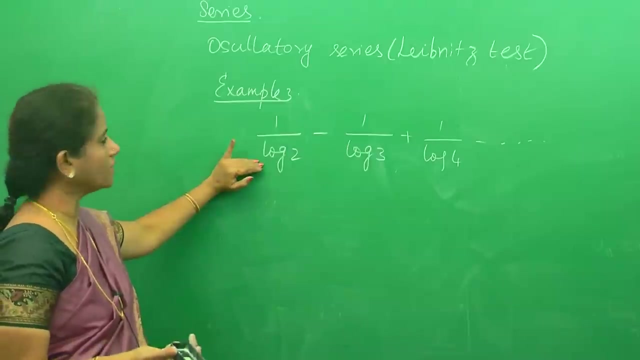 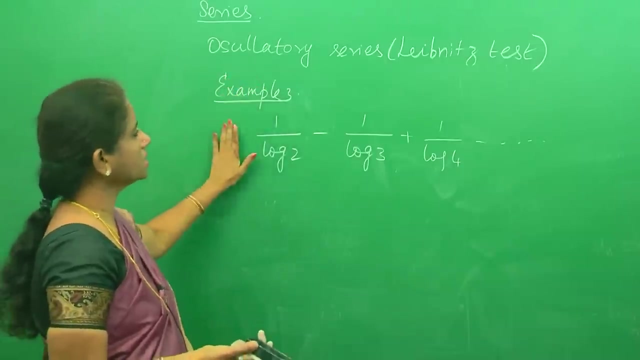 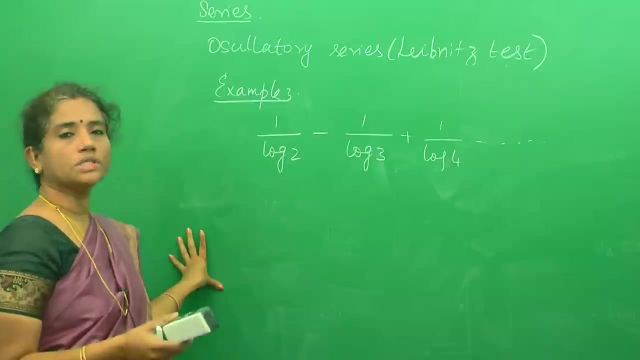 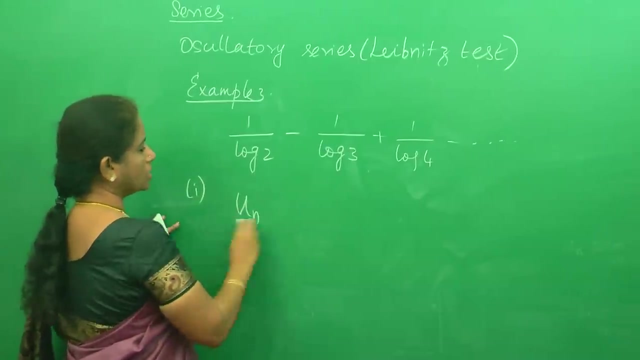 check the convergence of 1 by log 2 minus 1 over log 3 plus 1 over log 4 minus, etc. okay, basically, you know, log 2, log 2, log 2 value will be smaller than log 3 value and because it is in the denominator, I know it will satisfy the Leibniz test. and remember all the questions we did in Leibniz series is sorry, using Leibniz test is each term is positive, negative, it is alternating. basically, Leibniz test is used to check the convergence of an oscillatory series alone. okay, so now let us write u n, which is the first step. what is u n? 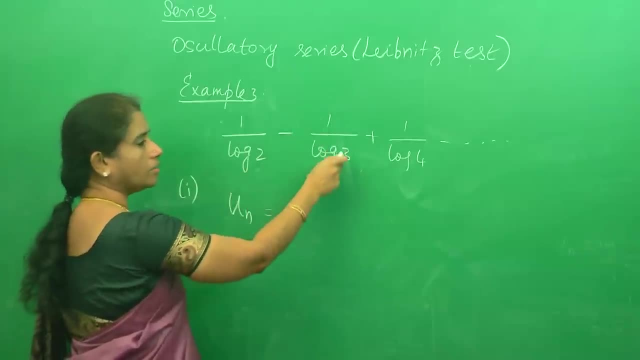 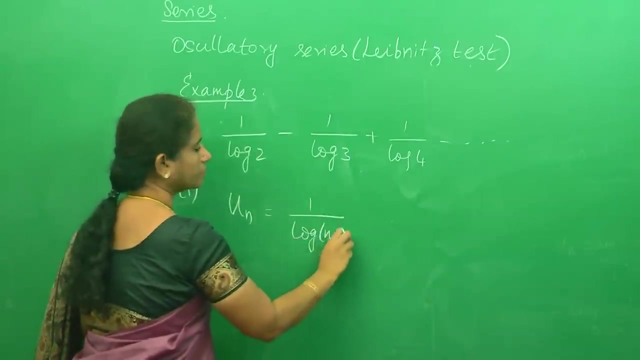 first term is log is here. second term is 3 here, so 1 by 3rd term means 4. so nth term means n plus 1, means 1 more than the term. first term means 2. second term means 3th. third term means 4, so n th term will be n plus 1, 1 more than that. 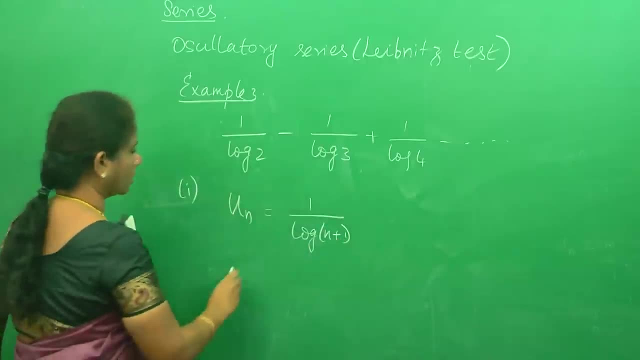 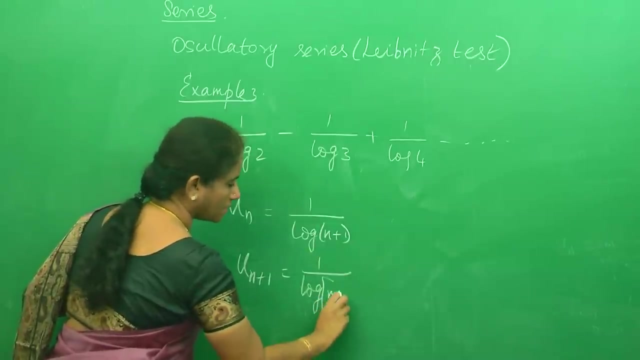 OK, and what is u? n plus 1? u n plus 1 is, as you know, n should be replaced by n plus 1, so this is nothing but one. the principal variable n, right? so we'll say this one. it's a зв value, So this is nothing but 1 by log of n plus 2.. 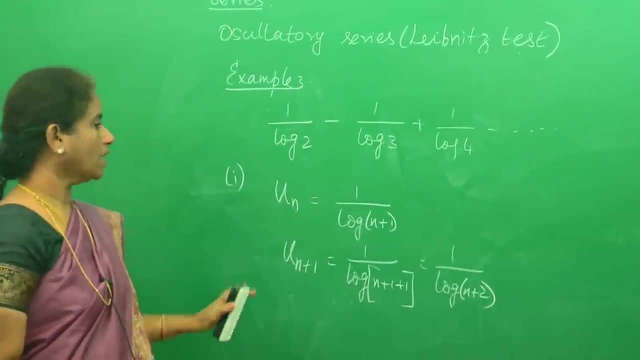 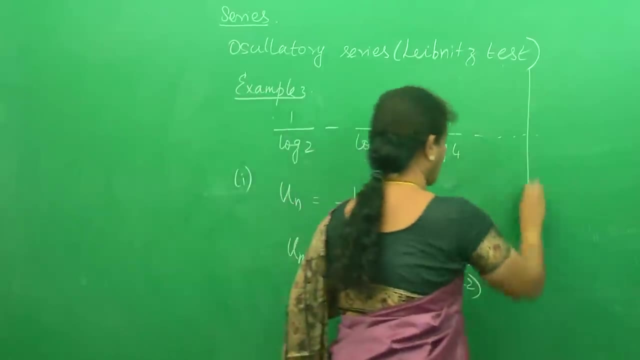 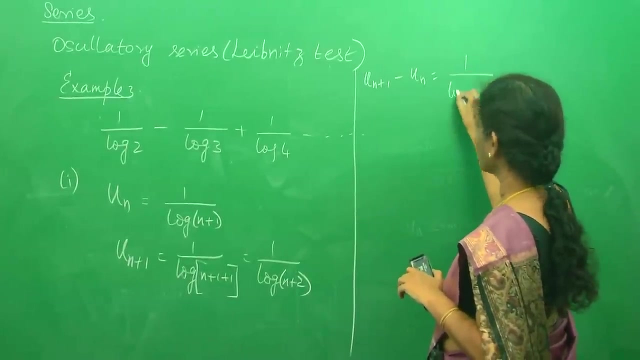 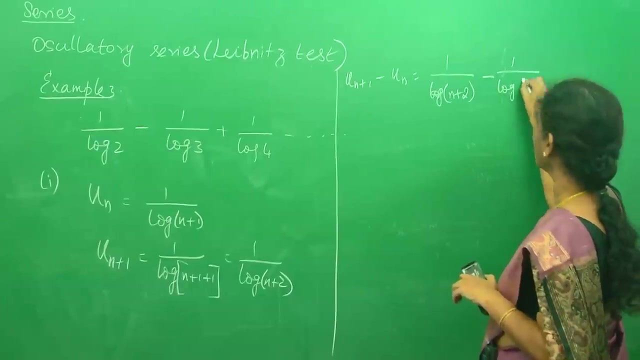 So we calculated un, we calculated un plus 1.. Now just I have to subtract and check whether it is greater than 0 or less than 0. So un plus 1 minus un is 1 by log of n plus 2 minus 1 by log of n plus 1.. 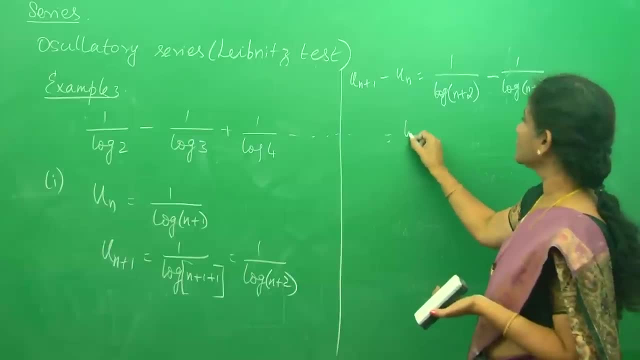 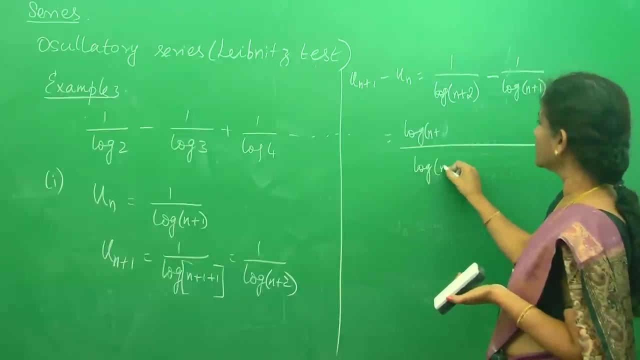 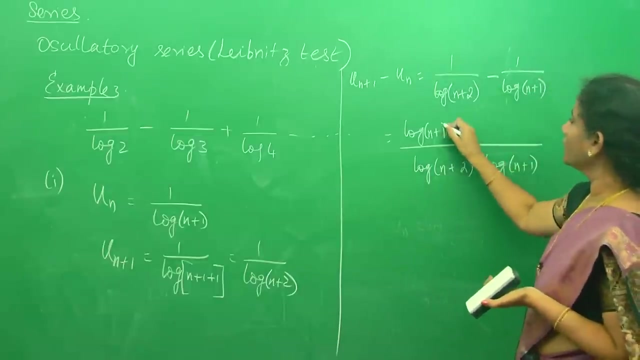 When you want to subtract them, you will take LCM. So this is log of n plus 2, sorry, the LCM is log of n plus 2 times log of n plus 1, and this is log of n plus 1 minus log of n plus 2 and the denominator is positive. 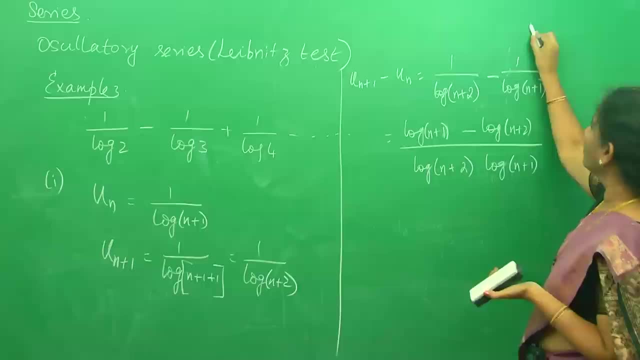 So we are going to check the numerator and you know log 2 is smaller than 1.. So log 2 will be smaller than log 1.. Basically, you know log 1 is 0, ok, So same way. sorry, it is not the same.